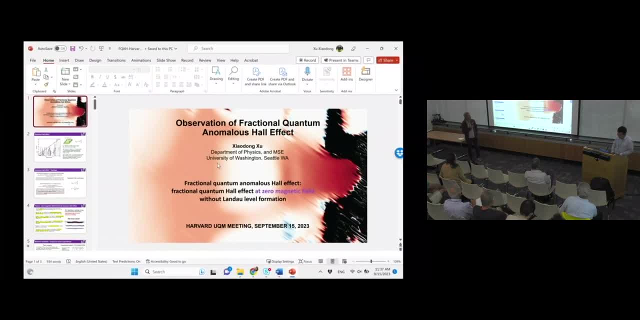 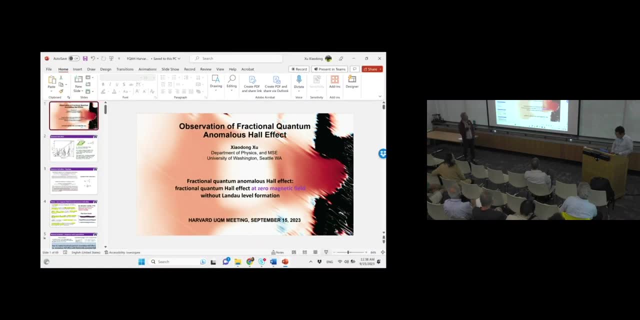 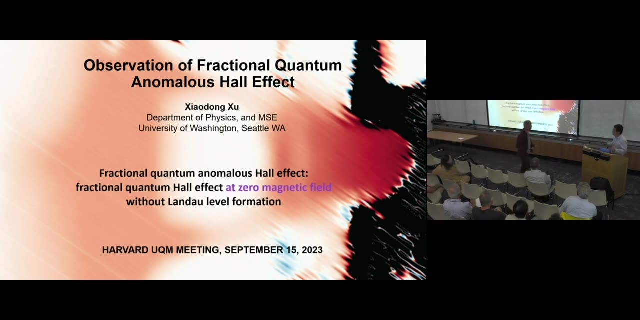 Okay, the second talk in this session is by Xiaodong Zhu from the University of Washington, And he'll be talking about observation of fractional quantum anomalous Hall effect. Do we have a microphone? Oh, sorry, I still have one. You can give a talk. 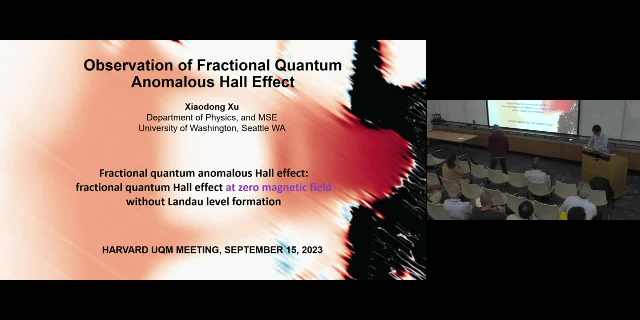 Okay, thank you. Okay, I would like to thank the organizer for the invitation and to this UltraQuantum Matter workshop. And today I'm going to tell you something I'm really excited about is this fractional quantum anomalous Hall effect. I'm going to call it FQAH. 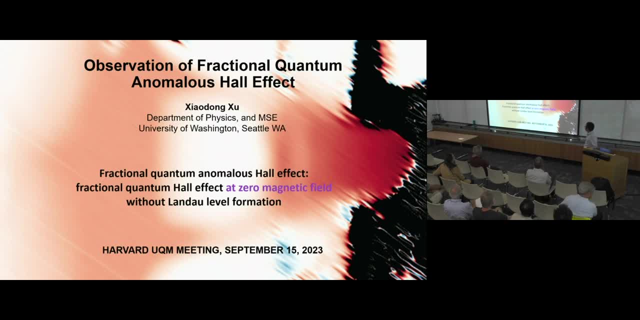 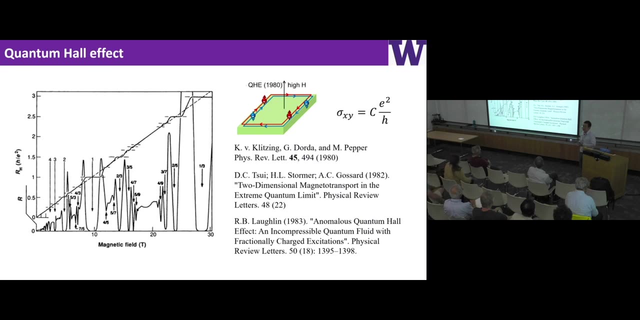 Just to define right this fractional quantum anomalous Hall effect is a fractional quantum Hall, as everybody knows, but a zero magnetic field and without the lambda level formations. So we know that the quantum Hall effect probably is a landmark discoveries in the condensed matter physics. 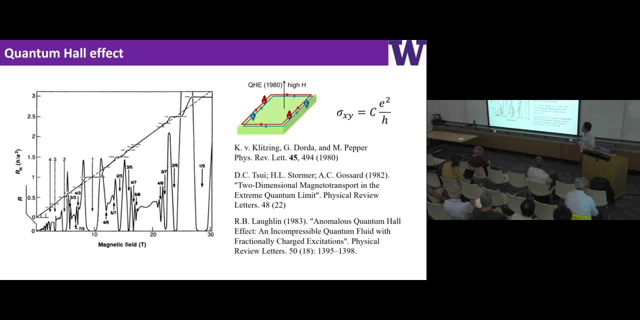 And this is just early data. you know from all these pioneering papers What they measure is Hall resistance, RH as function of the magnetic field, and you will see a lot of plateaus at the particular magnetic field, all the feeling factors. 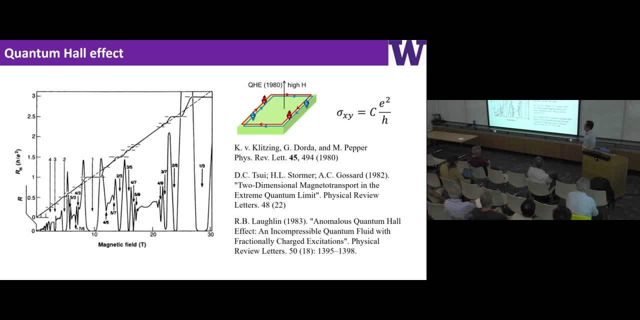 And what's really remarkable is that these Hall conductance is, in a particular form, right C times E squared over H, And the C is the chain number. now we know that The reason. it's remarkable because we know the material itself right. 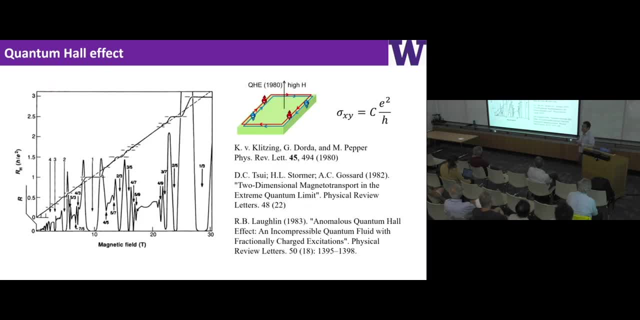 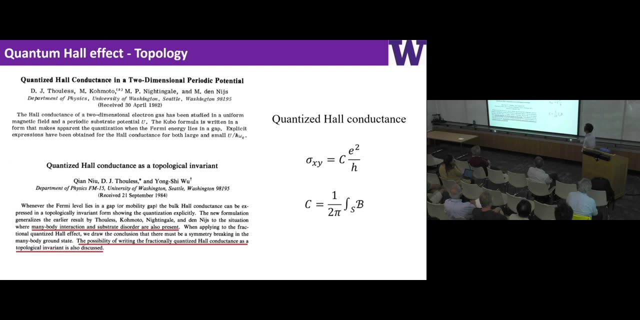 It's actually quite dirty systems, But these kind of collective behavior of electrons and show you that the resistance is quantized. Therefore, now we know that these remarkable phenomena is coming from the topology of the systems. As you know, my colleague David Paulus, 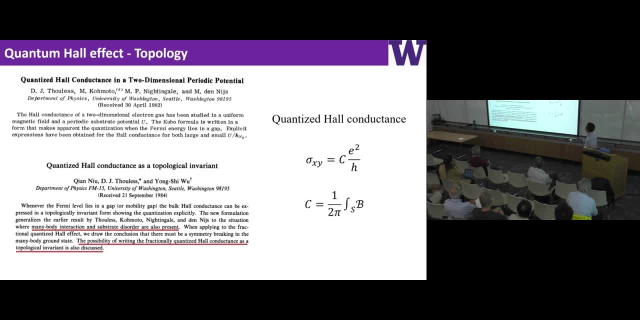 and his collaborator right back to the 80s, they showed that these systems and the chain number can be defined by the integral of battery curvature in the unit cell momentum space. And later, I think a couple of years later, and Chen Liu Solis and also Wu. 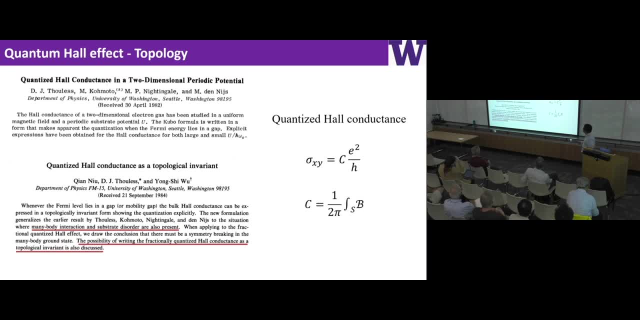 they come up with another paper. I think quite exciting is that they show basically extended the previous TK KM paper into the regime. The regime was mainly about the interactions and also with substrate disorders. So in this paper they're basically able to show. 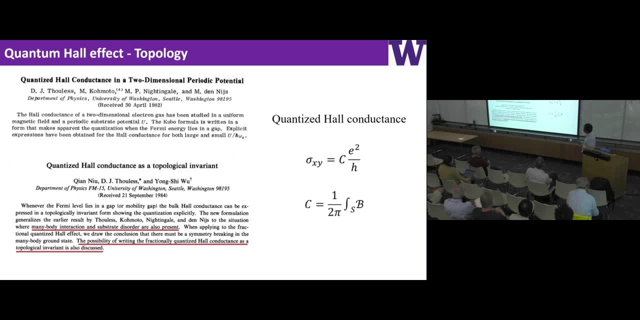 that the fractional chain number also is a topological invariant And in this particular paper- I think the time when they did this calculation- there's no dependence on magnetic field, Although I don't think they also realize fractional quantum number saw effect, but they don't consider magnetic field in this particular paper. 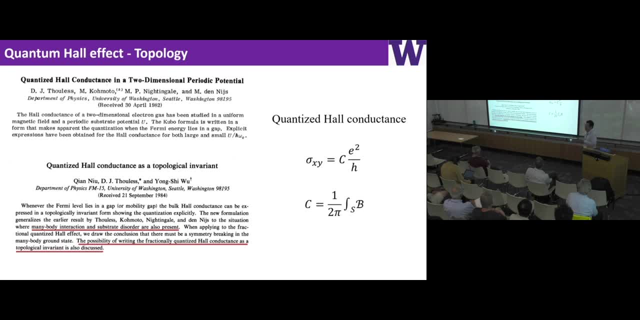 So now the question is: how can we then realize this kind of quantum how effect of zero magnetic field? And Duncan Hoden, right, he come up with this trial model back to 1988, and it shows that the integer quantum how effect. 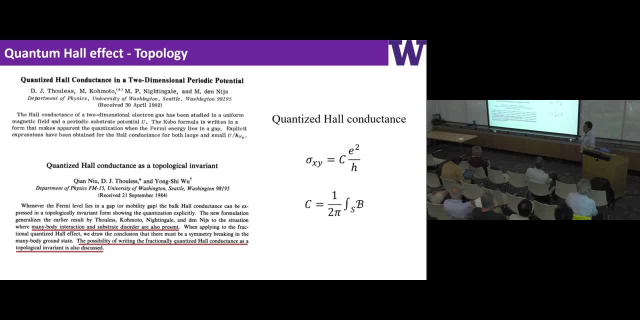 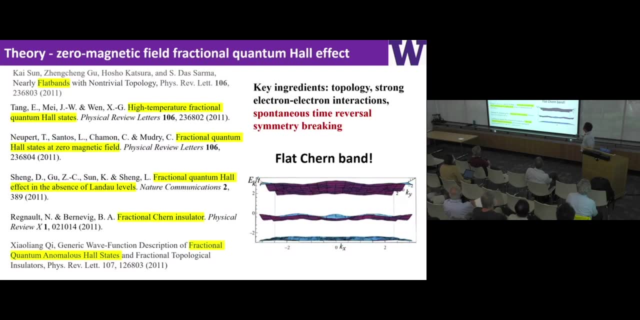 actually can be realized in this Hanukkah ladder structure, And Monica talked about lots of these effects we call quantum how effect- The zero magnetic field version of a quantum how effect actually be theoretically established much later in 2011.. So there's quite a few papers. 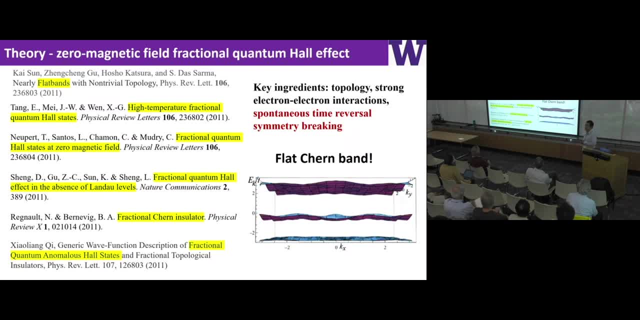 which discuss how you can realize these fractional quantum, how effects at a zero magnetic field, or you call it fractional chain ladders. So key ingredients for this effect is you need a topological band, you need a strong electron-electron interactions and also you need a spontaneous time reversal symmetry breaking. 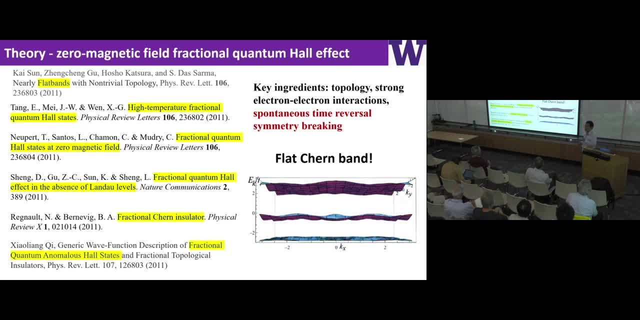 because we're talking about zero magnetic field And one key element to realize all these ingredients is that we need a flat chain band, And the only theory paper is that they basically propose. you know, you can realize such a state, but it doesn't point you into a particular material system. 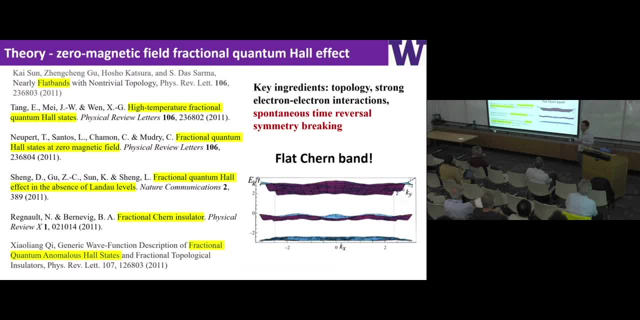 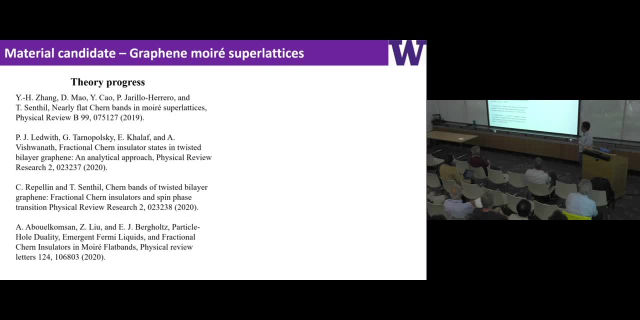 So there's a lot of theory work being proposed, like all kinds of material systems. Relevant to my talk is Lisa Murray's superlatives, and Monica already gave a pretty good introduction on the materials. I think the motivation is coming from right. 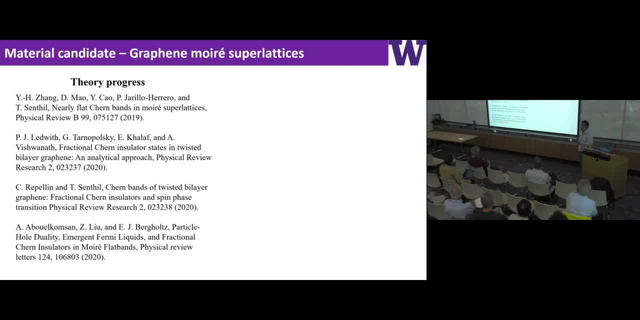 Pablo's, his landmark experiment shows that in this twisted graphene you can engineer these unconventional phenomena right, more than just superlatives, I think. So people got motivated and there's a theory, work, you know from Harvard, from MIT, right. 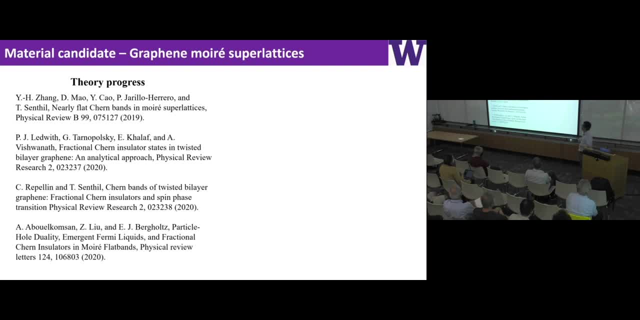 also shows that this effect is a fractional quantum and also effect actually can be engineered in these Murray's superlatives. In all these theory work they point into these graphene Murray's superlatives because that's the system when the wind was hot. 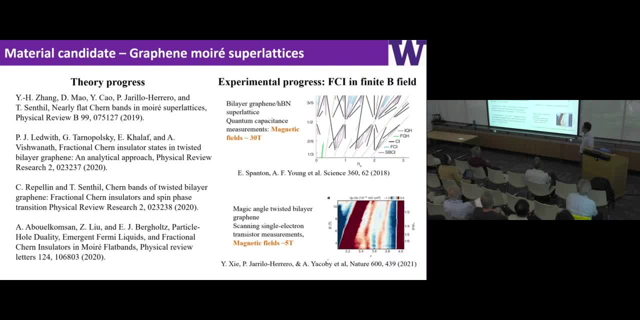 Indeed there's a quite a few exciting progress. So shows that fraction change later, but in the presence of a magnetic field. So the first book is from Andre Young's group. They study the Murray's superlatives formed by bilayer graphene and HBN. 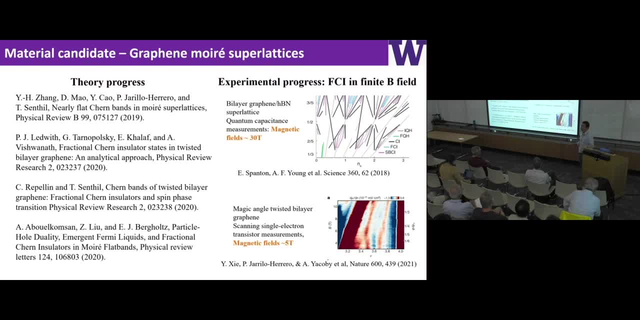 They found these fraction change insulator states in the presence of above 30 Tesla of magnetic field. And then the collaboration between Pablo and also Amir. they also show that in match angle, twisted bilayer graphene, these FCI states actually can exist at the low magnetic field. you know. 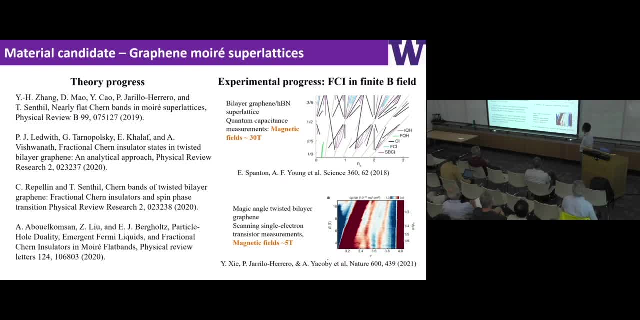 roughly they show up, start about five Teslas. So both experiments actually establish thermodynamic evidence of these FCI states, but in the presence of magnetic field. Then we go back to the same question, right? How can we realize this FQH state? 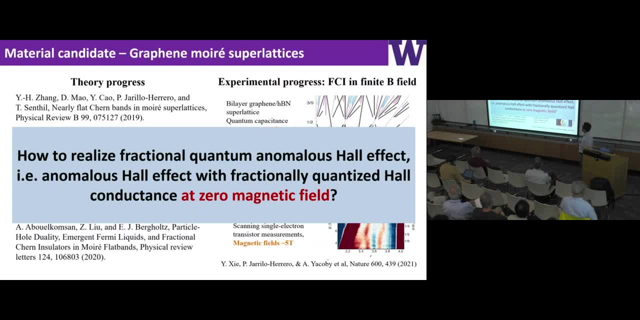 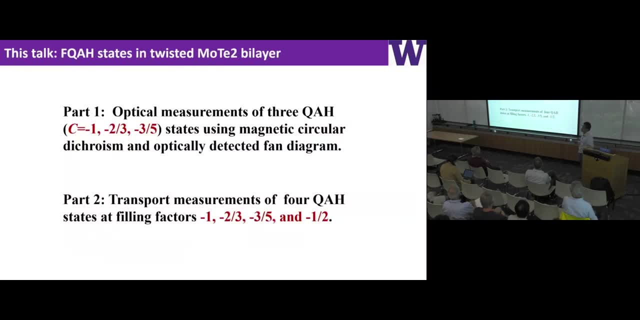 which is- I think it's a non-Luss-Hull effect, but it was a fractionally quantized Hull conductance at the zero magnetic field. So what I'm going to tell you today is that we can realize these FQH states. 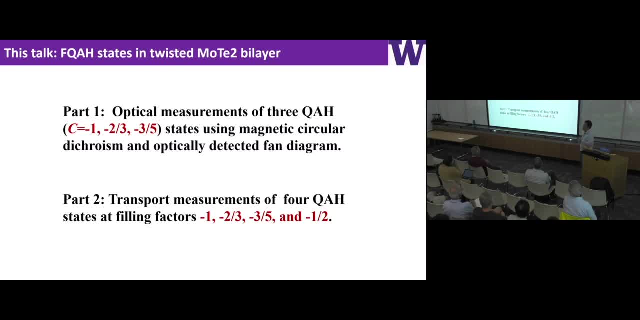 in the twisted MOT2 bilayers. And then my talk has two parts. The first part I'm going to show you are optical measurements of the three quantum anomalous Hull states with chain number minus one, minus two-thirds and minus three-fifths. 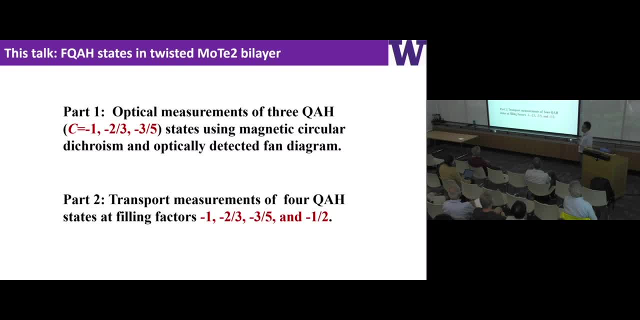 Use these magnetic diacrism measurements and also use optically detected fine diagrams, And then in the second part I'm going to show you the transport measurements. so we pretty much show the same states, but except we see another new state at minus one-half. 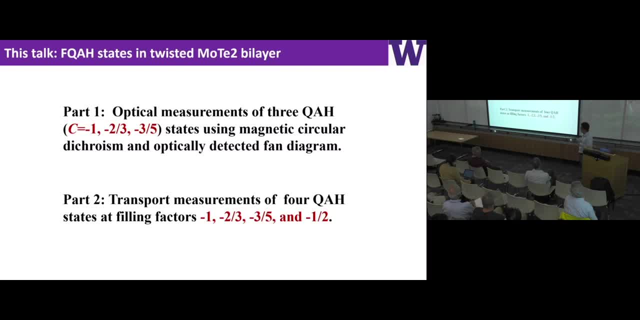 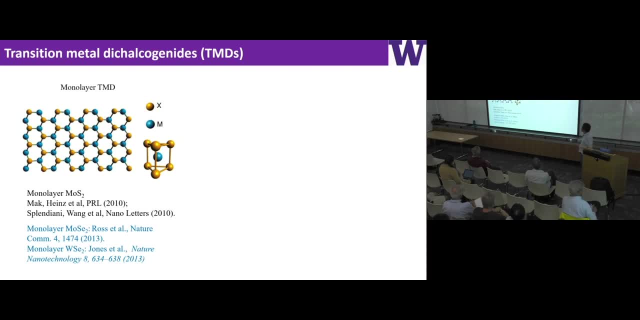 I'm going to tell you why we can't see in the transport but not in the optics. Okay, So just briefly. the material system we use belongs to the transition metal dichrogenites. The famous one is MRS2, right Discovered by Tony Haines and Feng Wang. 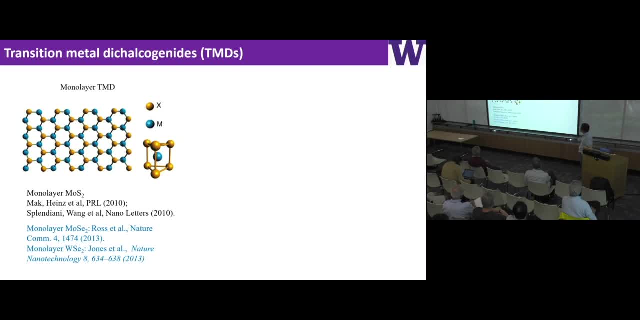 back to 2010.. So in these monolayer TMDs, if you look at these crystal structures from the top, they form this honeycomb-like structure and with a and a metal on each of the corners. so the break is an inversion symmetry. 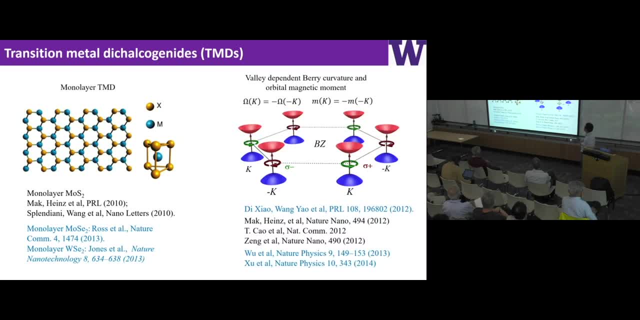 An important consequence of these inversion symmetry breaking is that give rise to these valley-dependent barrier curvature and also orbital magnetic moment, proposed by my collaborator Di Xiao and Wang Yao. So this effect actually is a valley-dependent property from the foundations for the for this topology physics. 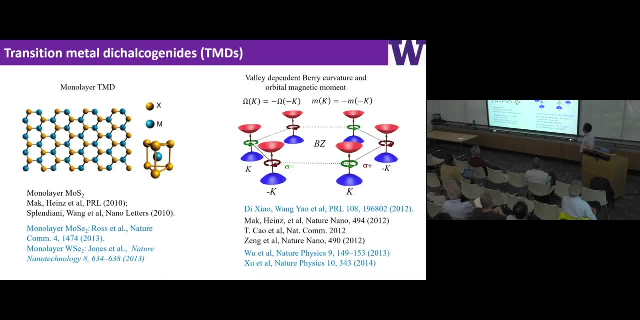 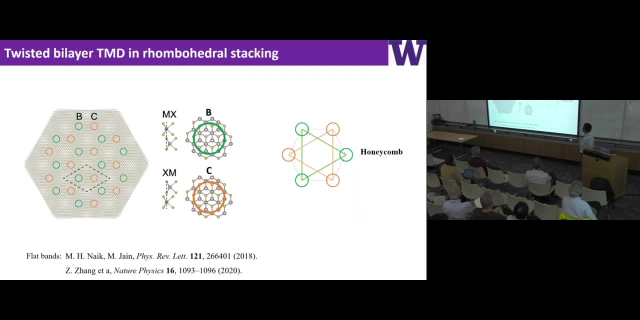 I'm going to tell you. So: imagine, right, we take one layer of this TMD and the stack on top itself. then we form a bilayer, but with a little twist. So this is called rhombohedral stacking. to supply this: 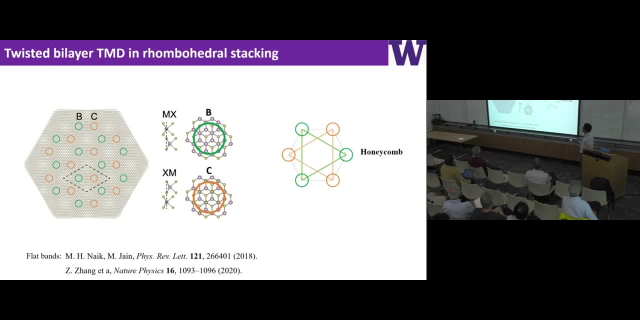 So in this type of AA stacking structure there's two energy degenerate minimals. in a moray lattice There's a, B and a C. So B is with a metal on top of coctrin and the C is coctrin on top of metal. 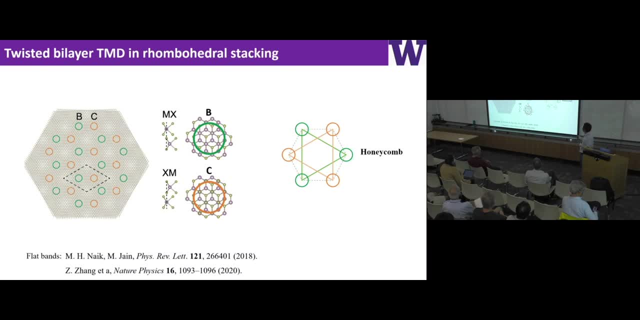 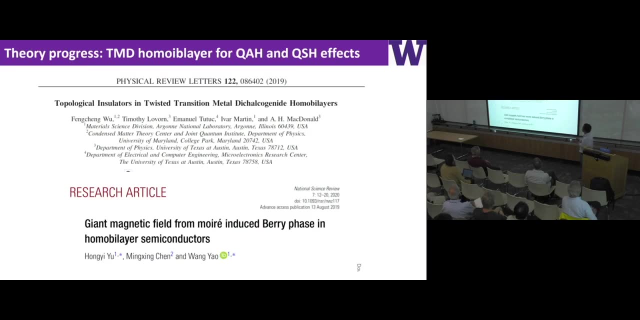 Then these two sublattices. they form a honeycomb lattice structure Back to 2019, right, these two papers already showed that in these TMD homo bilayers you can study topologic physics. So yeah, the first one is from Allen's. 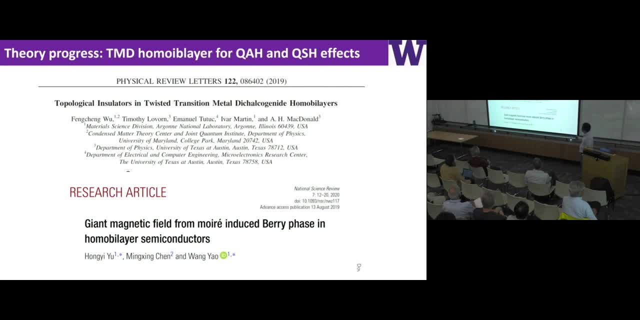 and the second is from, like my collaborator Wang Yao, Both papers actually study the twisted MOT2 system. So our work actually just started from there because my collaborator Wang, he told me you should work on these materials, Even though at the time, 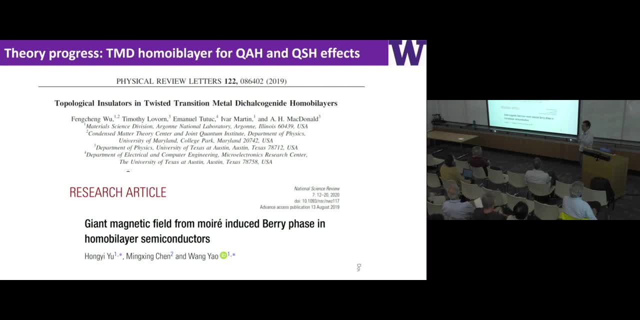 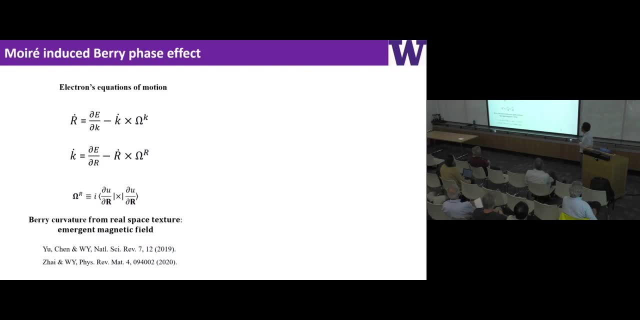 he doesn't know there's a fraction and quantum number states in this particular system, but he knows it's topological, at least based on the theory. Let me just briefly go through the theory in one slide and give you kind of an idea why the system is topological. 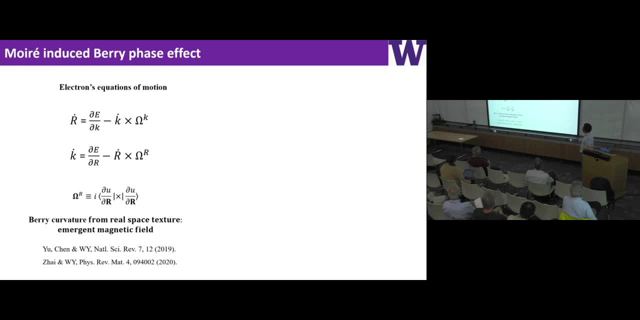 So if we look at these electrons' equation of motions- right, we have the two terms. So the first term is about positions, right, You can see that there's an omega k term and in the second part is omega r. So omega k is the barrier curvature. 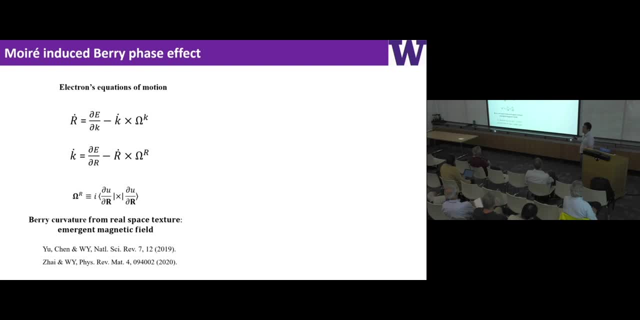 in the momentum space right, equivalent to a magnetic field in the momentum space. And the second part is actually it's the barrier curvature effect in the real space. So usually for the single crystal we deal with, it's a homogeneous crystal. Therefore this term of this omega r. 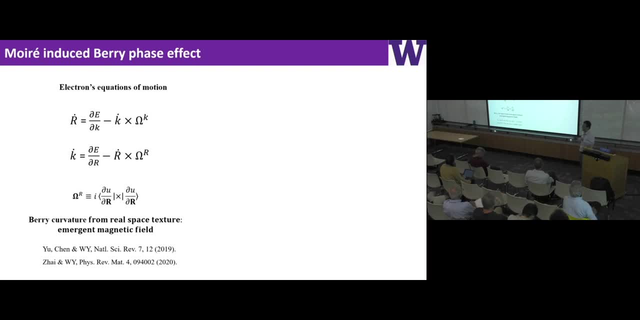 which is the barrier curvature in the real space. it's ignored. We don't have it right, because the crystal is homogeneous. But then the situation changes in this moiré sublattice, So let me just walk you through it. 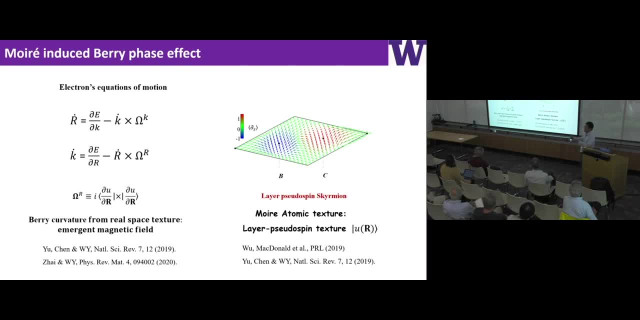 I told you we have two moiré sublattices, B and C, which are energy degenerate. B is with metal on top of collagen, C is collagen on top of metal. Then you can imagine if I start to evolve from. 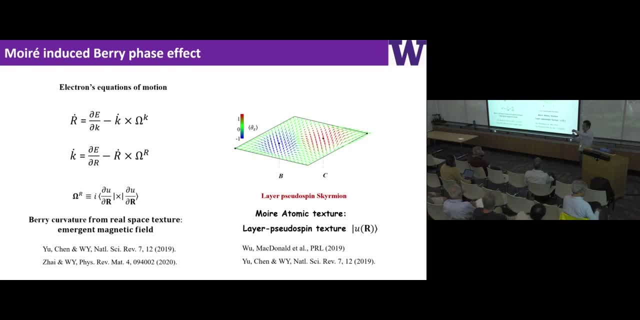 you know, move the position from B to C, then this local atomic registry must change right. Then this forms these moiré atomic textures And you can also- you basically can- consider these as a layer, pseudo spin textures And in Alan's paper, 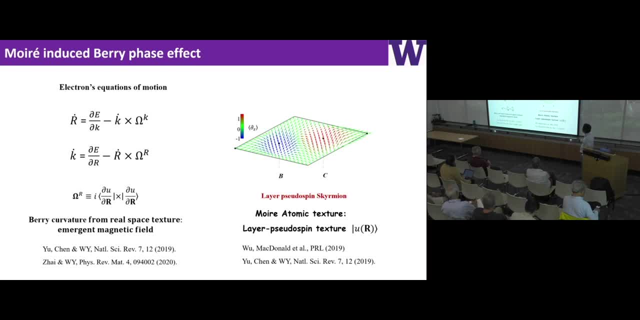 basically shows that these are layer pseudo spin skirmishes. So we know, if there's a skirmish in a real space, then you have this real space barrier curvature and give rise to this emergent magnetic field. So this, this is the original topology of these. 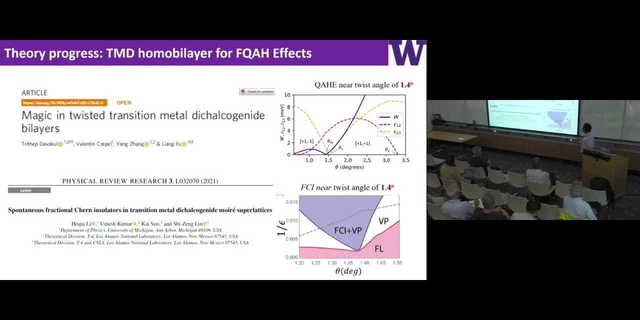 homo barrier systems. We started working on this material back to 2019, but you know I'll have to tell you initially it doesn't work, So my students all got discouraged. Then there's another two paper come out. One is from Liang-Fu's group. 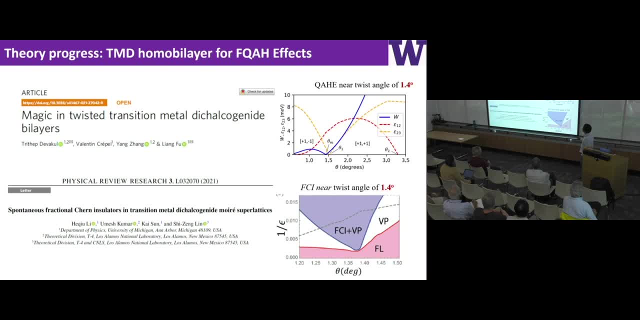 They study the twist of WSE2.. And it shows that there's a corner, anomalous Hall effect, a twist angle of about 1.4 degrees and also with indication of this FQH state And the other one is more relevant. 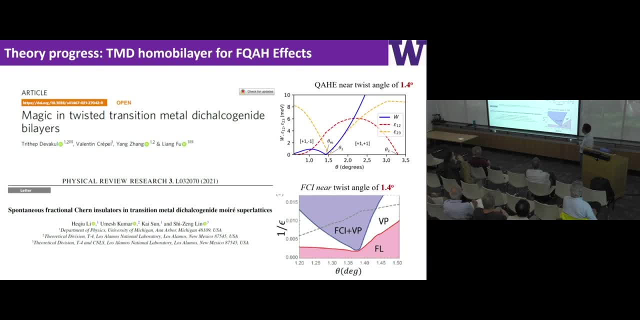 It's from the collaboration between Kai Sun and Shi Zhenglin, ETL. What they show is that the MOT2 systems- actually they did this mini body calculation- They found this chain number. Basically you can, you can have this fraction chain insulator state. 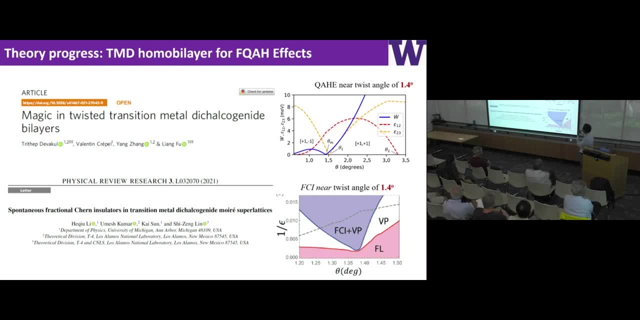 You have a twist angle of 1.4 degree as well, just consistent with Liang's calculations. Then my students got really motivated because now I have two more papers right. They showed me that indeed there's something exciting, And it was twist angle 1.4 degrees. 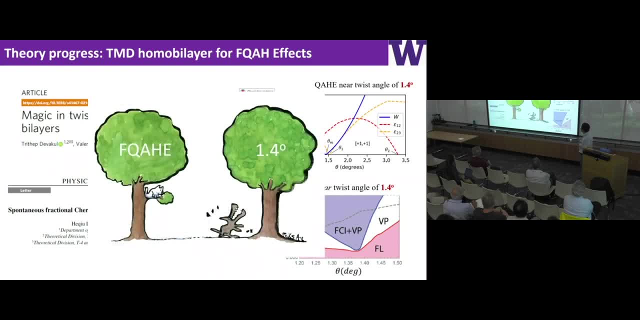 So we started working on these systems for about a year And it turns out well, we're just like this little puppy. Actually, 1.4 is not a right angle. Then my students got discouraged again. Then I told them: okay, 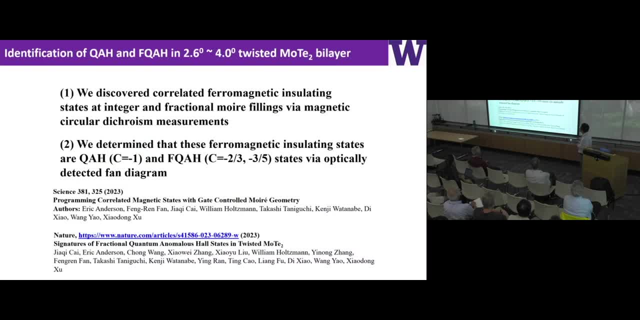 well, forget about this 1.4. Let's just try something, right? So this we're going to tell you today- And you know the initial twist angle- what we found- actually what's working- is random, right. 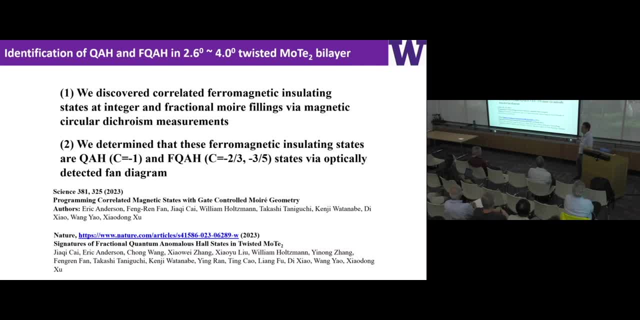 It's around like 3.5 degrees, 3.5 to 4 degrees. But now you know we test a lot more devices And the others also in the community test a lot of devices. I think the range we can safely say. 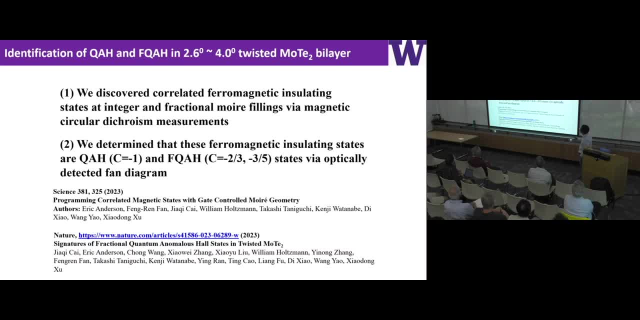 have these QH and FQH states is between 2.6 to 4 degrees. But this range I think it's dynamic range. I think with more and more device made, probably the range will also be expanded. But the take-home message is that 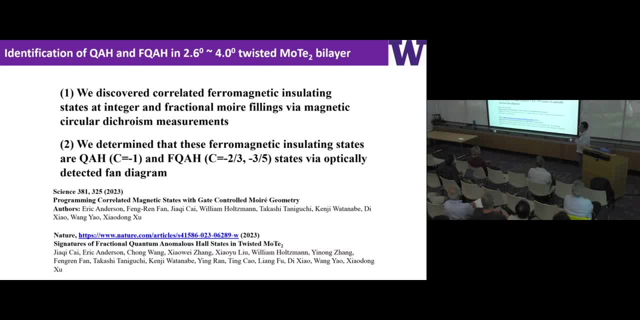 actually it's not as very sensitive to twist angle. The twist angle is large, Okay, But it's not 1.4.. It's just a joke, It's not offensive joke, Okay. So anyway, I'm going to tell you is that? 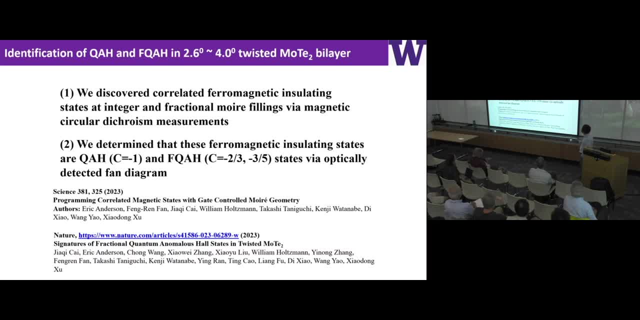 we discovered these correlated ferromagnetic insulating states at the both integer and the fraction Mori fillings. Use these magnetic dichroism right. We need a spontaneous temporal results image breaking. The second part is then. I'm going to show you how we can use optical technique. 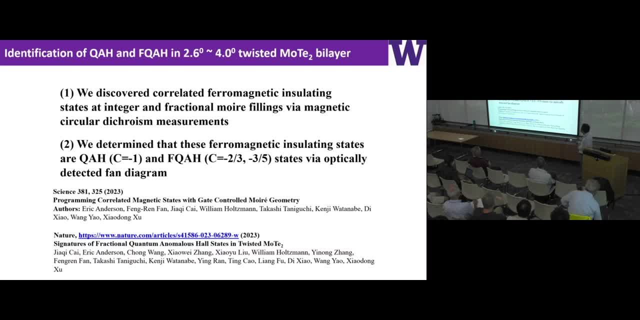 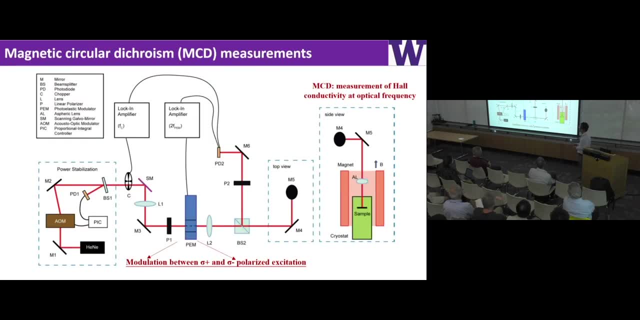 to determine these quantum anomalous state. The details can be found by looking at these two papers. So I know a lot of theorists sitting in the audience and I want to scare you with. this diagram is how we measure this dichroism. There's a lot of components. 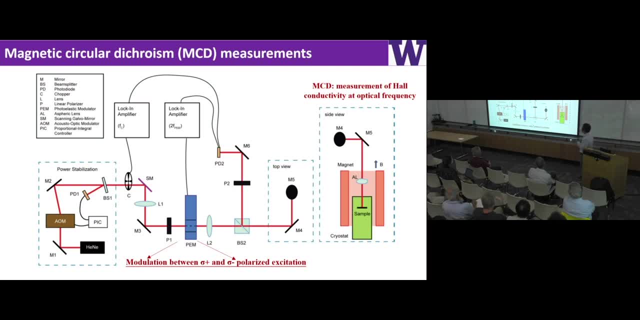 The only reason is here is try to scare you. The only the important part is the bottom part. I'm not sure if you can even see it. Is we basically sending laser beams and then modulate it between right circular and the left circular porositions? 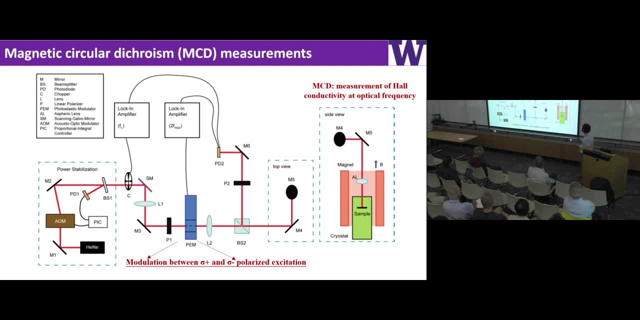 Then we send these polarization module light to a sample. We measure the reflection difference between left and right circular porositions. So we call MCD, which is a magnetic circular dichroism, So MCD measurements, if you're not familiar with it. 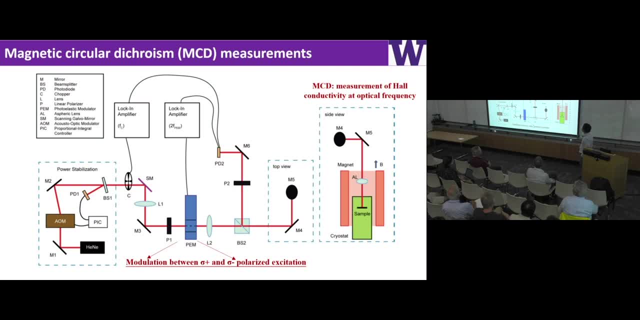 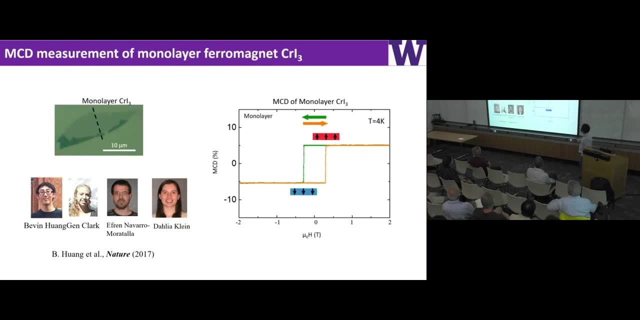 you can think of it as a measurement of the hall conductivity, but at the optical frequencies. Okay, So that's all I'm going to tell you. Then we're going to use this MCD technique. Here's just one example what the signal look like. 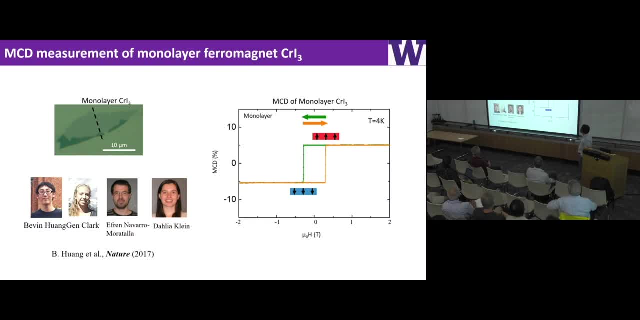 And this is what we measured many years ago on this monolayer ferromagnet, in collaboration with Pablo's group, And what I show you is that the MCD signal as function of a magnetic field sweeping up and sweeping down. So there's a key features right. 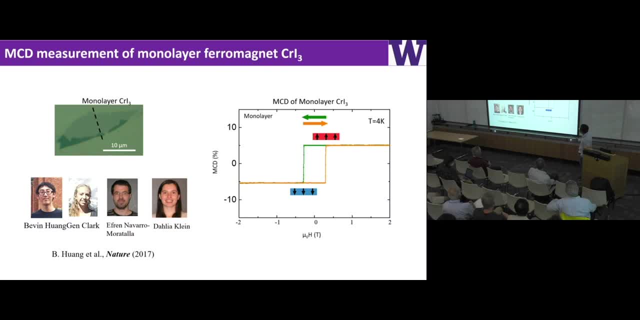 You see there's a finite MCD signal at the zero magnetic field, And then also you see a hysteresis loop. So all these are hallmark of a ferromagnetism in a monolayer. Then we perform the same measurement. 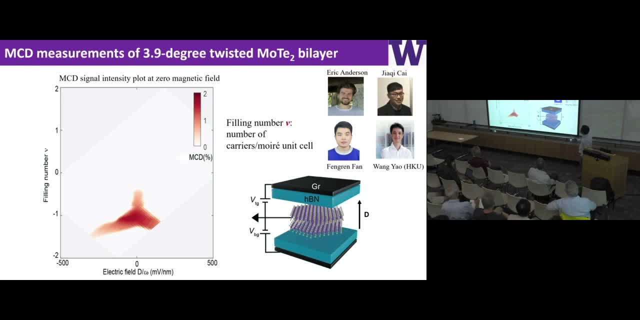 The data I show you is from 3.9-degree twisted MOT2 bilayers And here's a schematic of samples. We have a dual data structure, Means we can control doping the sample. We can also control the perpendicular light field across the samples. 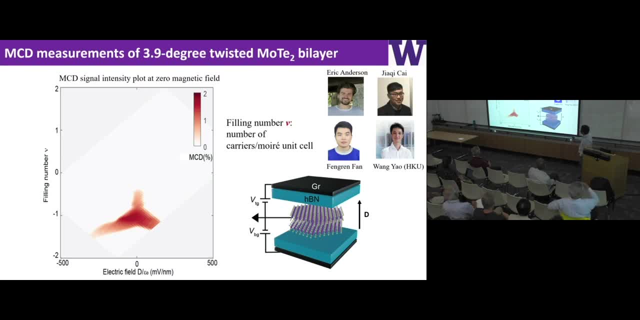 So in this diagram the vertical axis is the filling number, Means the number of carriers per monolayer cells, And the horizontal axis is the electric field. And you can see that in this large phase space, only at the whole doping site that we have this non-vanishing MCD signal. 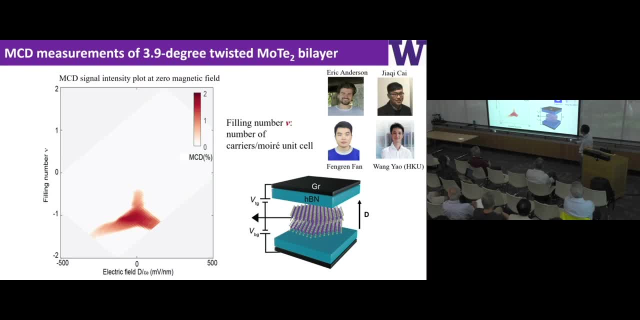 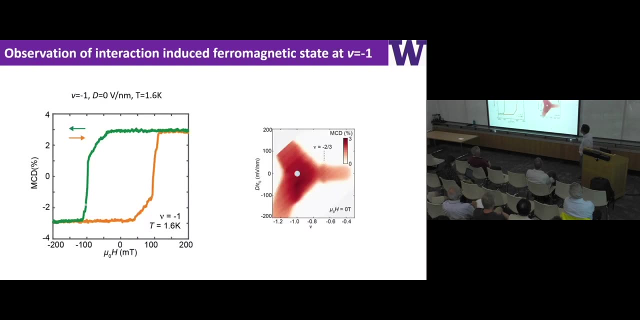 which suggests we have a ferromagnetic state at this phase space. And there's also two features here corresponding to the fraction filling and also integer fillings. And just to confirm, we do have these ferromagnetic states. I picked a spot in the phase space. 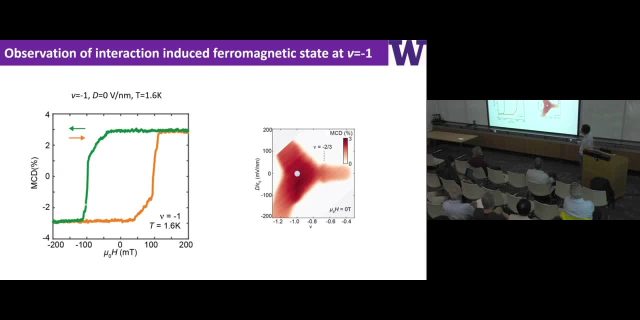 But the integer fillings. Then we can perform these MCD measurements as function of magnetic field. You can see, it is a Hiss-Rhesus loop, As I already told you, which is a hallmark of ferromagnetism. We can also measure these MCDs. 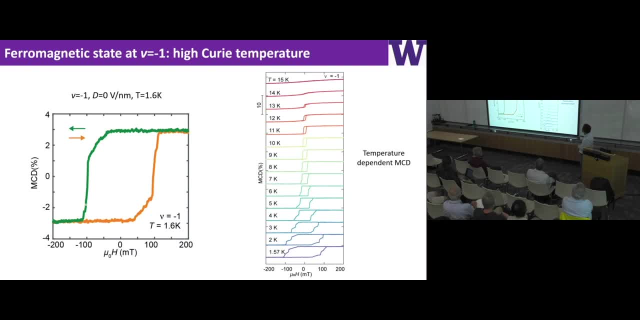 as function of temperatures, And you can see the Hiss-Rhesus vanishes as we raise the temperature. So the current temperature of the system is about 14 kelvins. It looks like not too high. right, It's a low temperature. 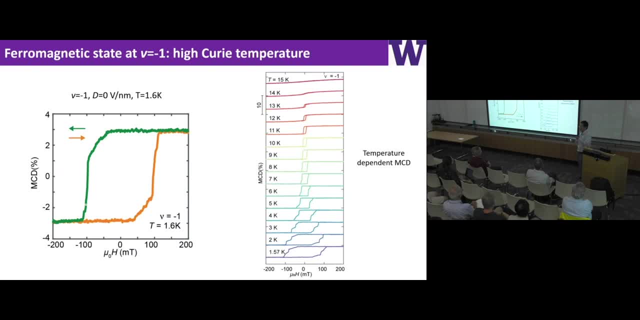 But actually, if you think about it, it's really high temperature, Because my moray unit cell has a wavelength of about five nanometers And the filling factor is one. It means there's one carrier every six or five nanometers of unit cells. 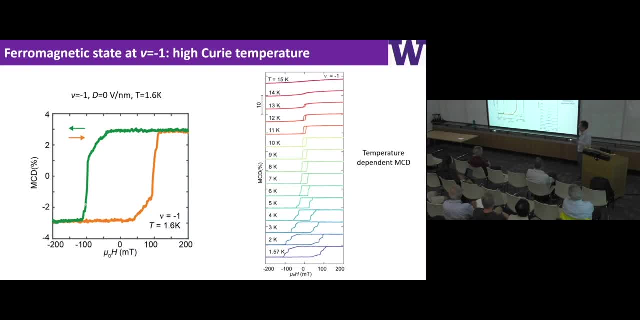 And the carrier density is really low. The spin density is very low And it's also in the two-dimensional, So the carrier temperature is actually 14 kelvins. So this already indicates something unusual in the systems. Then the next question is: 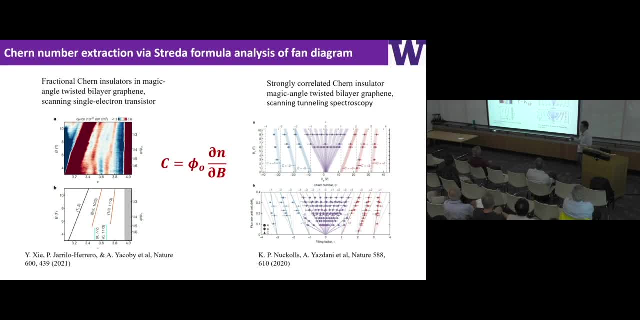 how can we measure the chain numbers? Initially, we cannot do transport, So there's two ways to measure chain number. One is just to transport If you can. If you cannot, then you just measure the fan diagram and use a strata formula. 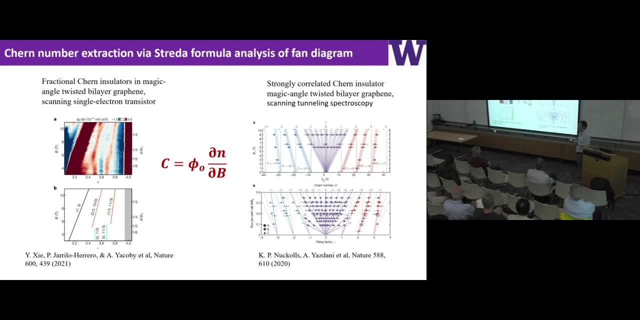 to fit this dispersion curve. So look for these thermodynamic evidence of the states. So here are just two examples. You look at the density of the gap states in the S-function magnetic field. So this is from Amir's paper. They look for these chain numbers. 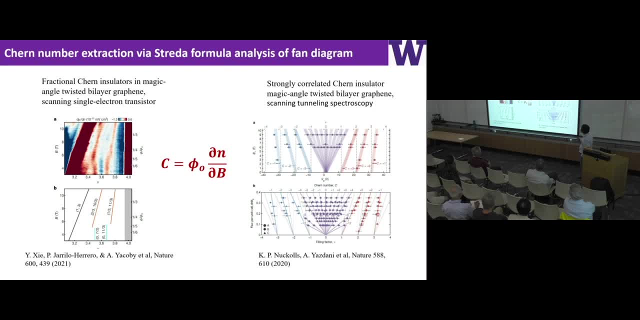 from these fractional chains, like states, And the other example is from Adyastani. They do STM right, which you cannot do transport. They also look for this dispersion curve to determine all the chains later in magic angle: tristagraphics. 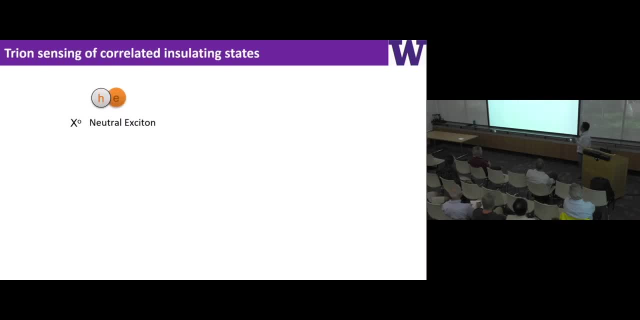 So we can use the same trick. But the probe we use is we call triumphs. So just give you a brief instruction. what is triumph? If we shine light to a semiconductor right, you create an electron-hole pair. They bond together. 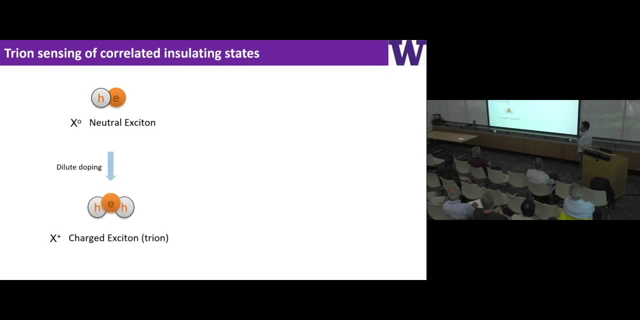 They form an exciton. So this is neutral. But if we dope the system, say I dope with holes, then these excitons are going to bond to an extra hole. They are going to form a three-particle system. So this is called triumph. 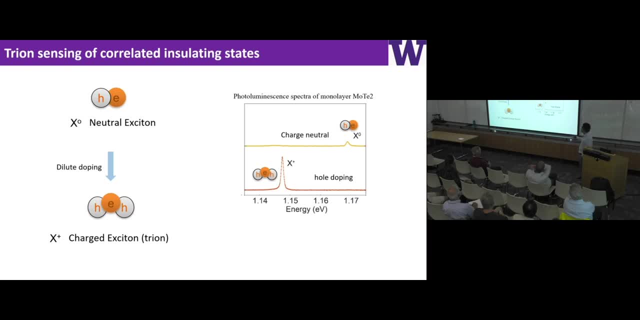 Here is a typical spectra- photoluminescence spectra- from a model in MLT2.. And you see, we have a neutral exciton emission and we have a charged exciton emission. You can see there is energy separation between these two. So you can clearly tell. 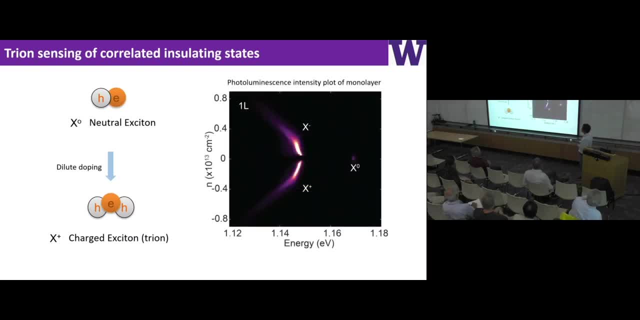 where there is a triumph formation. If I continually tune my carrier densities in this vertical axis, what I show you here is luminescence intensity plot. from a monolayer You can see a neutral exciton at the charge of neutral. Then you see triumph appears. 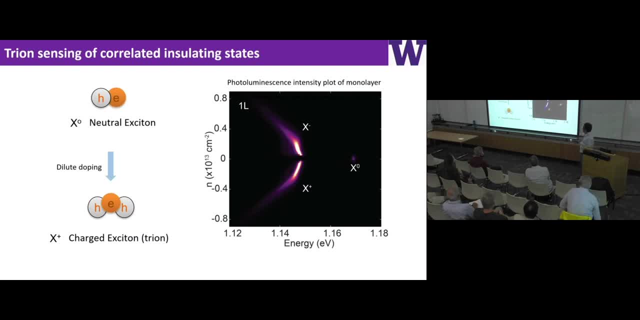 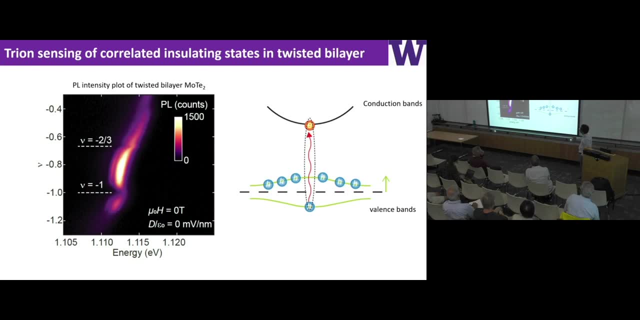 The intensity is sort of continuously tuned. Okay, Now, what I show you here is actually is a triumph intensity plot as function doping. or I already converted to feeding factors, but for a twisted value in MLT2.. Then in this plot you will see that there are two kinks. 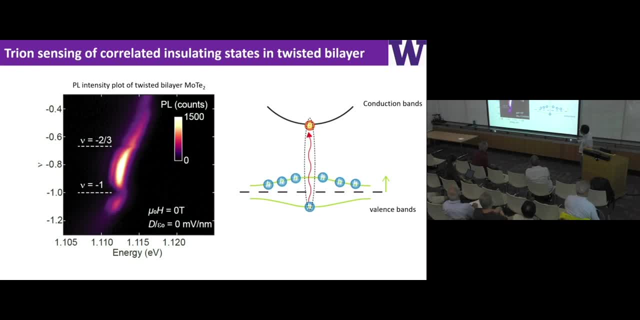 in terms of feeding factor. The first kink points to these minus two-thirds feeding factor, the second point to minus one. So these two kinks, you see the triumph: luminescence actually drops, the intensity drops. So the reason is that 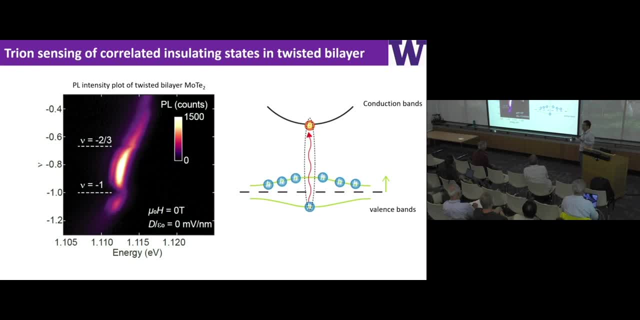 as I mentioned to you at the beginning, triumph is exciton bound to a free carriers. But in a system when there is a correlated state forms means there's a gap state form, then the service, subfamily service, is gapped. The number of free carriers to form triumph. 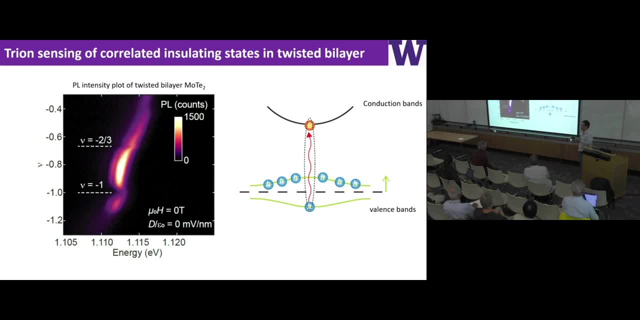 actually is reduced, So you can think of the number of triumph also going to be reduced. Therefore, the luminescence from the triumph will also be reduced. So what do we do is that we're basically looking for the reduction of the triumph luminescent population. 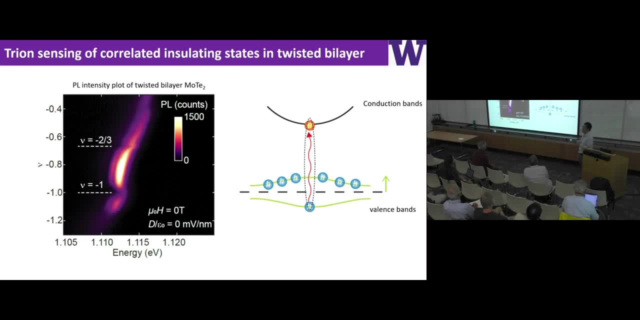 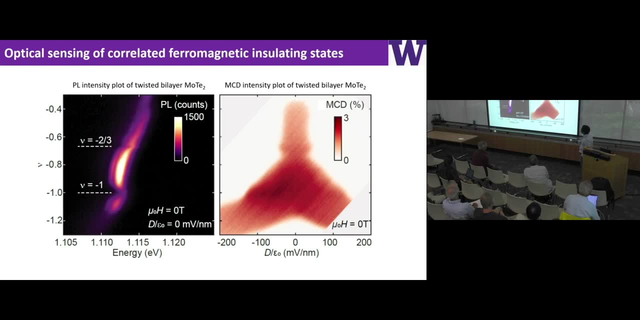 This is a signature of the formation of a gapped state. Then we can compare this luminescence intense plot to my MCD measurements. You can clearly see whenever there's a gapped state we see there's sort of an enhancement in the 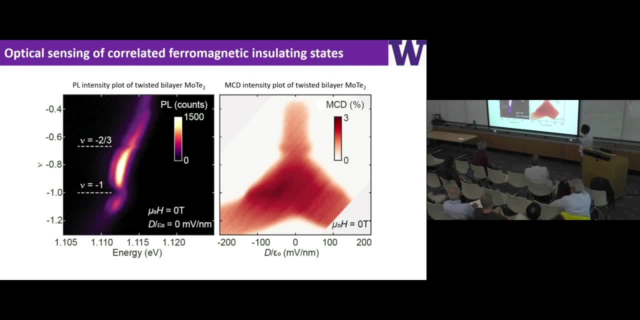 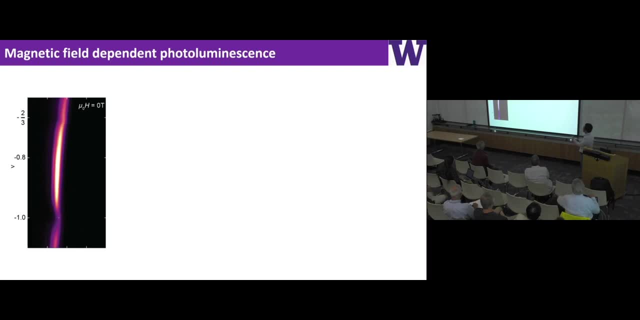 we have this little bump for this MCD signal. So from this kind of comparison we can establish we have a ferromagnetic insulin states. So next step is then we do the same measurements but at a different magnetic field, So from zero Tesla all the way to four Teslas. 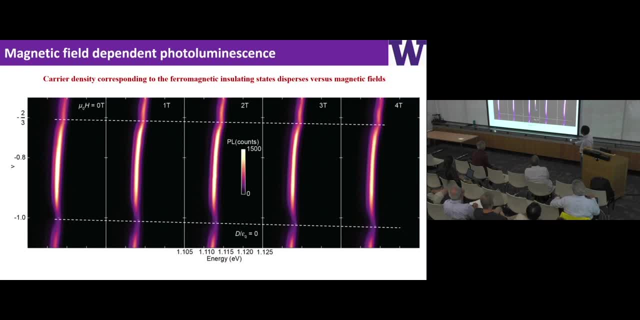 And if you look at the carrier density, for example, correspond to this magnetic field, you will see that actually it changes as far as the magnetic field. Basically there's dispersions. So this tells us there's something actually topological, But this is very not quantitative. 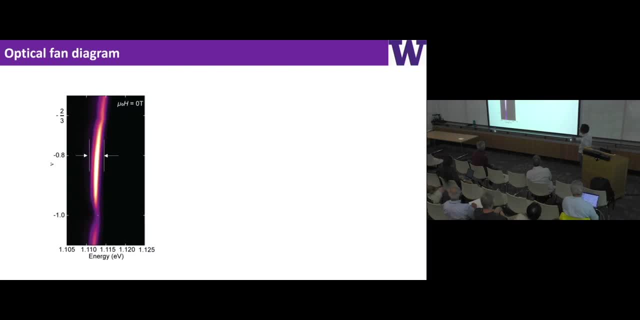 To do some kind of a quantitative comparison. what we do is that we perform a special integration of this luminescence right over these spectral windows. Then we plot this spatially integrated PL as function of feeling factor at the particular magnetic field, for example. 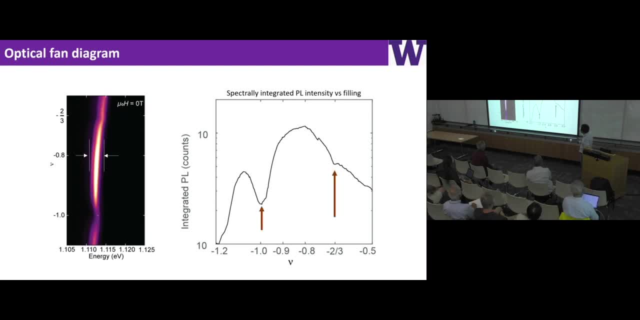 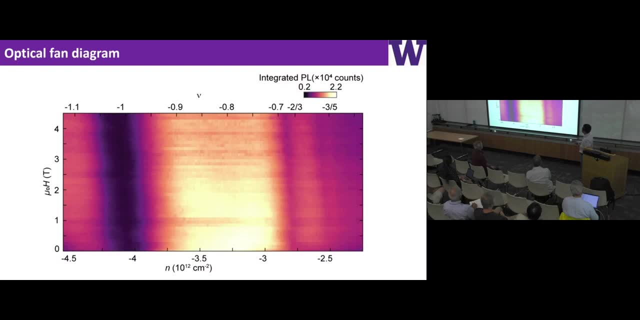 Then you will see there's two dips correspond to these two gapped states. Then I plot these line traces as function of magnetic field and get these fan diagrams. And in these fan diagrams you will see there's three features here: one, two, three. all right. 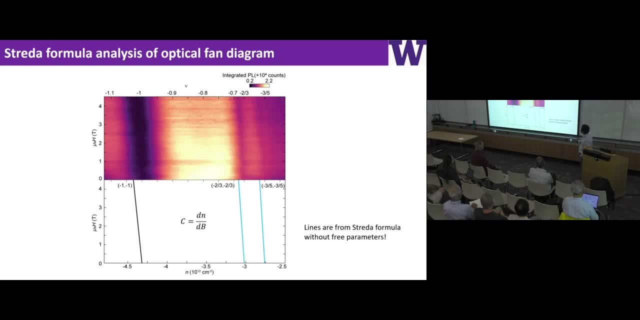 Then we can compare these three features with the dispersion compared to these strata formula analysis. So these are the three expected lines from these topological states And the first one where you can see all these lines actually can fit to my data really well okay. 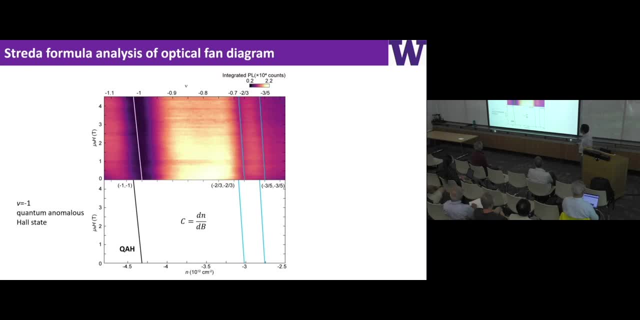 So from this comparison, what I conclude is that the state of the feeling factor minus one is a quantum anomalous half-state, and the other two are the minus two-thirds, and also minus three-fifths correspond to the fraction quantum anomalous half-state. 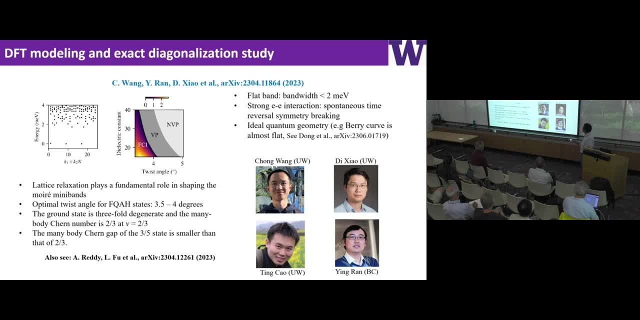 So these are the measurements we have. At the same time, my colleagues- you know my collaborator Di Xiao and also Liang Fu- they did independent calculations on this system to see whether the measurement makes sense, Because initially right. 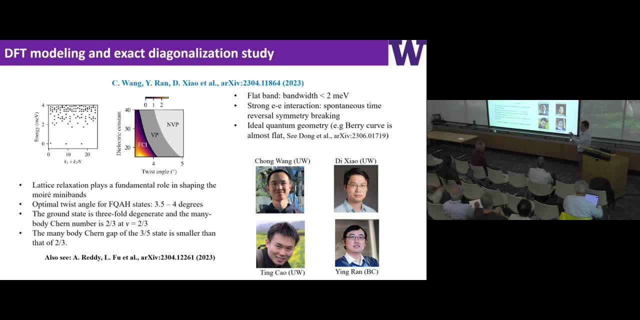 1.4 degree doesn't make sense. So they want to see what's going wrong, So both of them come up with similar conclusions Here. what I want to show you is the results from Di Xiao, And what we learned is that. 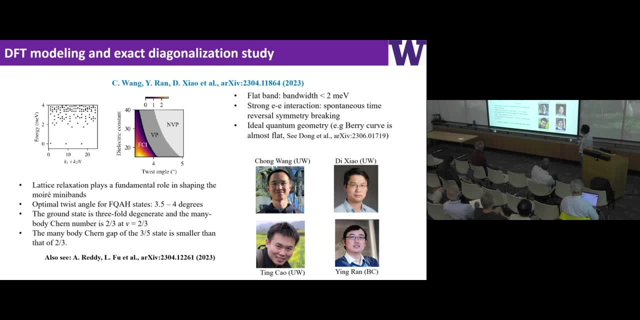 why it's wrong? because, well, what they found is that lattice relaxation actually plays a really important role to shaping memory minivans. That's how you determine the trace angle. So what he found is that for the optimum trace angle for this FQH effect, 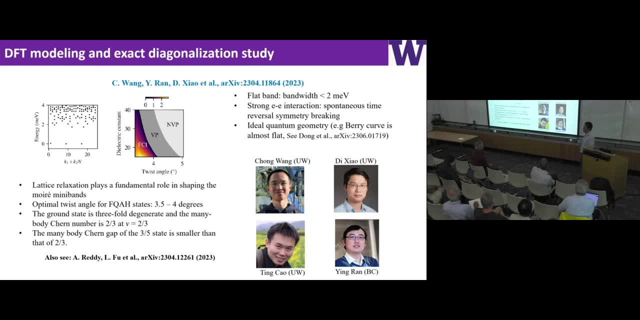 actually it's between 3.4 degrees. So we basically got lucky: make such a sample at the right angle. Then he also did a calculation to find these main body chain numbers. you know two-thirds and three-fifths, You know. he found these. 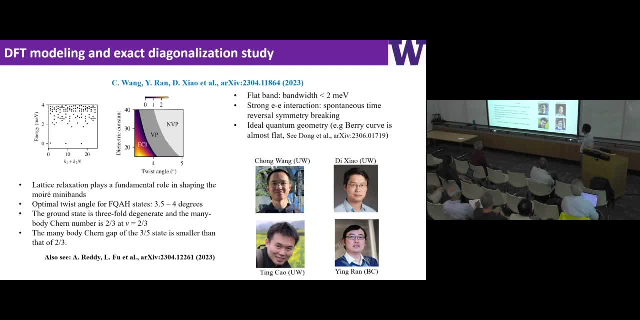 the gap from two-thirds actually is slightly larger than the three-fifths, So there's a lot of TMD system right proposed. I think a lot of people ask me what's unique about the MRT2.. So one possibility is well. 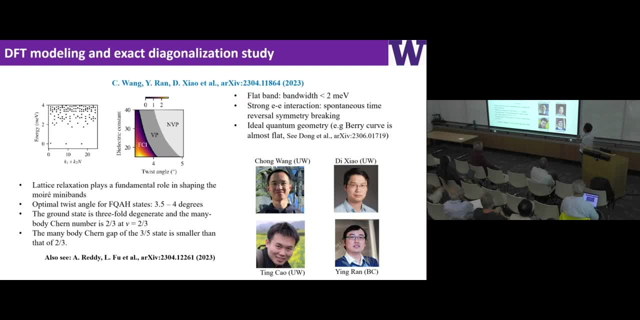 the band is really flat. So what it means is the bandwidth actually is smaller than 2 millivit. Just to give you a comparison, for magic angle graphene the bandwidth is on the other side. It's about 10 millivit. 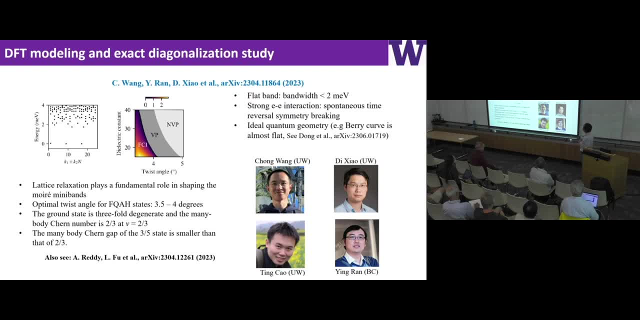 Okay, So it's already flat band right, But this is much flatter. The second thing is that there's a very strong electron-electron interactions give us these ferromagnetic states. And the third one is there's ideal quantum geometry. 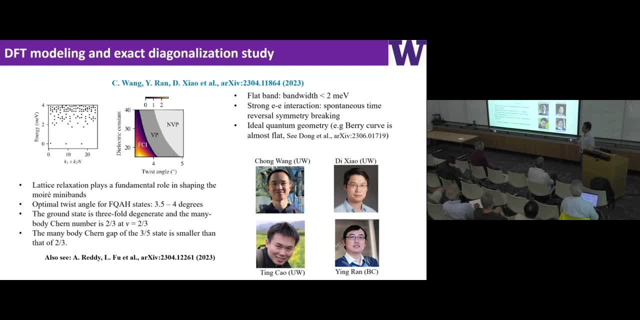 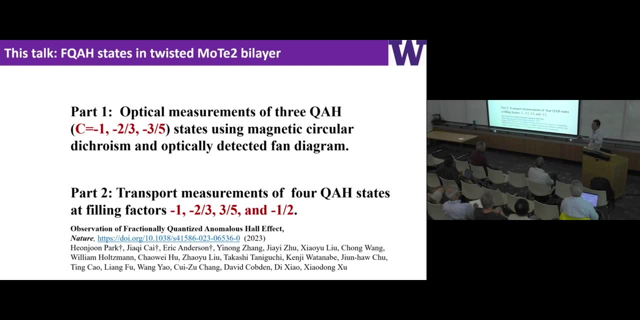 You know, you can see what it means from Ashwin and his collaborators' paper. All right, So let me see how much time I have. Okay, Not much time left, Sorry. Does spin orbital coupling play, though I would say yes. 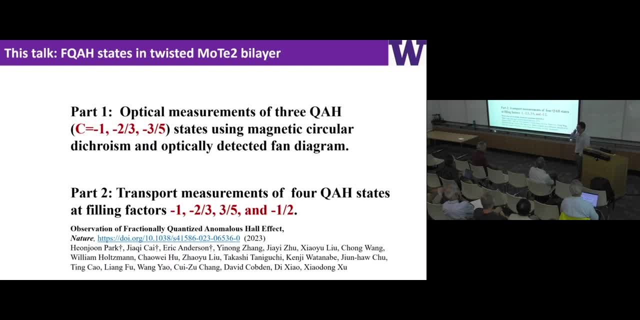 Yeah, Because this gives rise to these. you know the spin value locking effects in the TMDs. So part of them already take a lot of time, but I'm going to go to these part two, where the part one is give you a thermodynamic evidence. 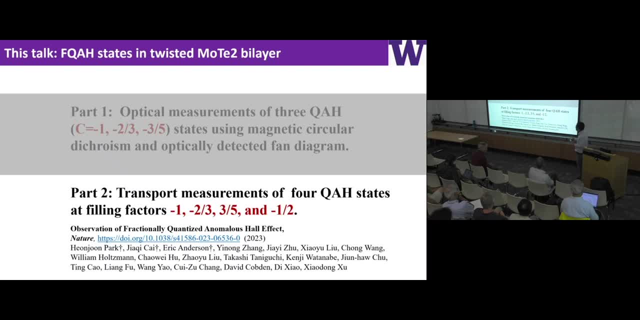 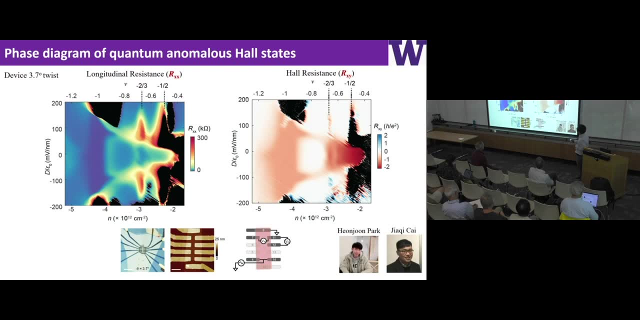 So the part two is where I show you the transport measurements. Here just one of the main results: right, We perform these measurements of these longitudinal resistance Rxx and also how resistance Rxy as function of a large field and the carrier densities in these plots. 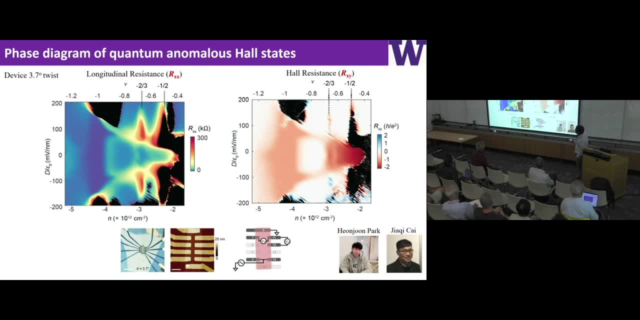 And there's a lot of things going on in these plots, right? You see, for example, the filling factor minus one, minus two-thirds. You see there's kind of a reduction, right Compression, of Rxx, But at the same time, 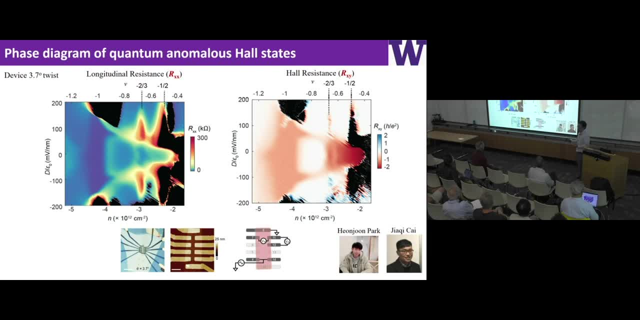 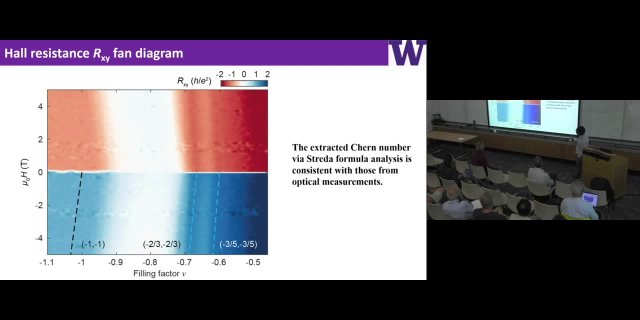 you will see enhancement of Rxy. So this already tells you, well, there's something interesting going on. So let's do a little bit of a careful study. So I took these Rxy measurements and applied it as function of magnetic field. 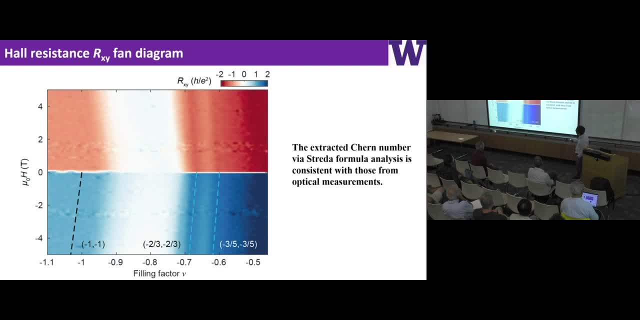 Basically it's a Vandegrang measurement And you can clearly see there's three dispersion features. And then we can fit it to this Strader formula. get the chain number minus one, minus two-thirds, minus three-fifths, And also, when you flip the sign, 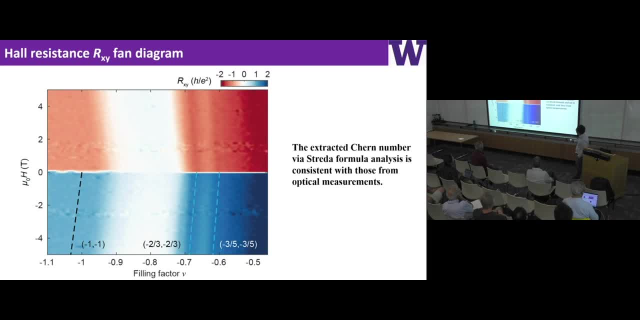 of the magnetic field and the slope right, The sampler slope also flips. This basically tells you it's not a quantum hot state. actually, It's a quantum anomalous hot state. So the take-home message of this kind of data is consistent with our optical measurements actually. 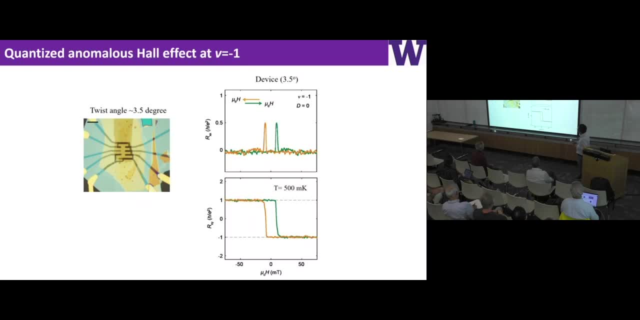 Basically it's the same measurements, just use different probes. Next is then we're going to do these magnetic field measurements. So the first is the filling factor minus one. You will see the Rxy is quantized at the edge of the square. 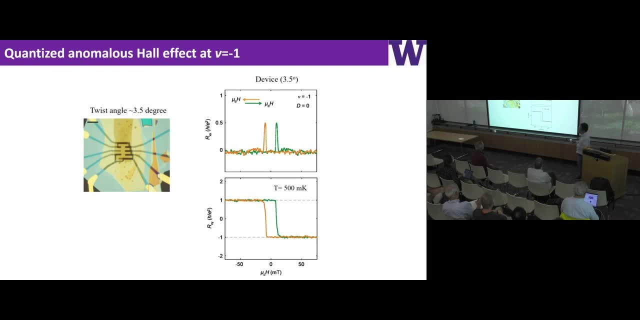 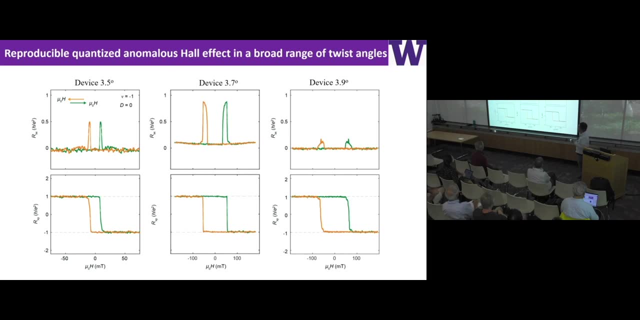 with nearly vanishing Rxx. And the zero magnetic field is precisely the hallmark of quantum anomalous hot effect, And we measured it in three different devices with different trace angles: 3.5, 3.7, and 3.9.. 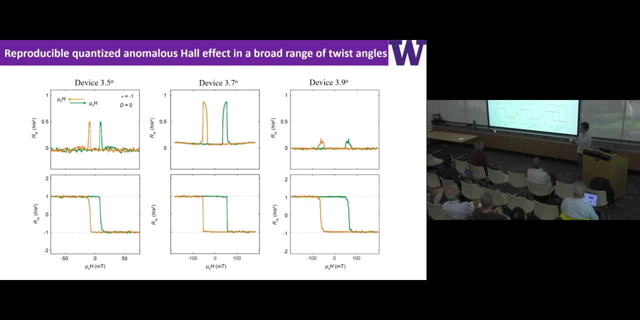 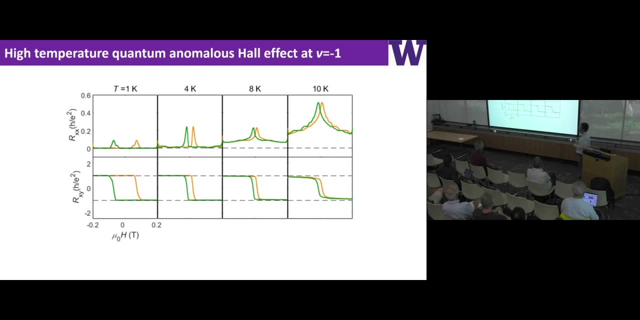 They basically show very similar behaviors. So the result, I think, is really robust. The nice thing about the system is that you can apply a large field to control these quantum anomalous hot states. One feature I want to show you here first is the temperature dependence right. 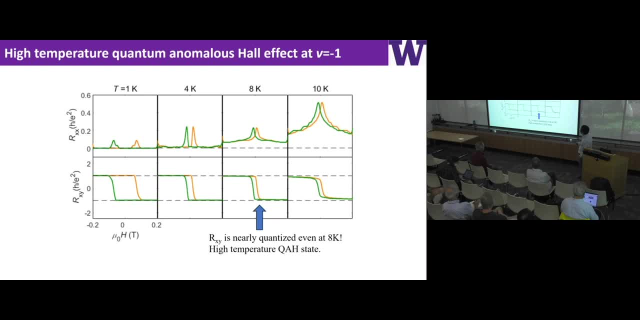 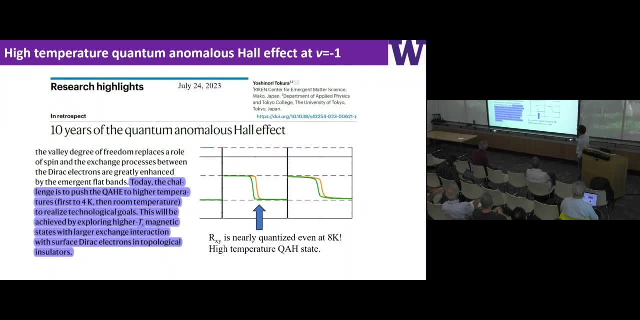 What I emphasize is that even at the 8 Kelvin, Rxy is still nearly quantized. You may not appreciate this number, so let me show you this paper from Yoshitakura. So we know that the QOH is initially discovered 2013.. 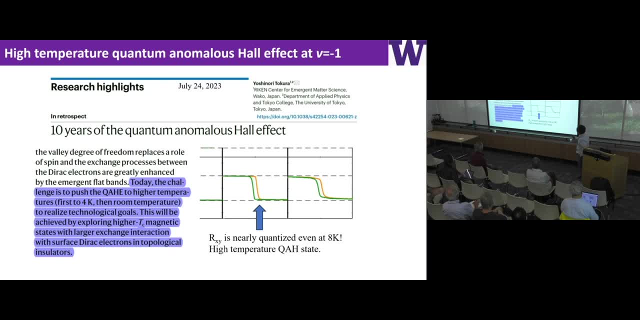 So this year is marked like 10-year anniversary. This is kind of a review article published about a month ago about this quantum anomalous hot effect. So what you see at the end, you can see. today the challenge is to push this QOH effect to higher temperatures. 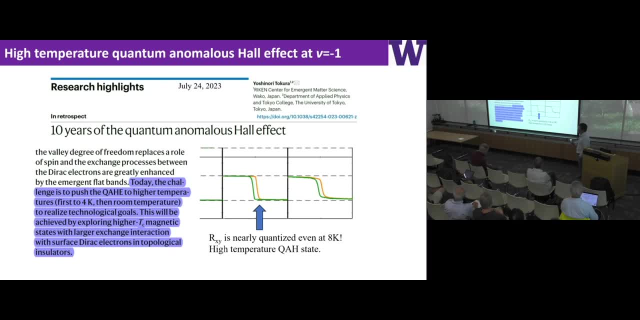 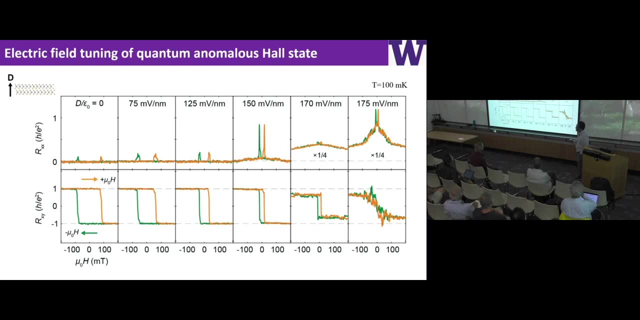 first to 4K, then to room temperature, And I think we probably already achieved this goal, at least the first goal. Then we can show how we can use a large field to tune this state. I think I don't have time. 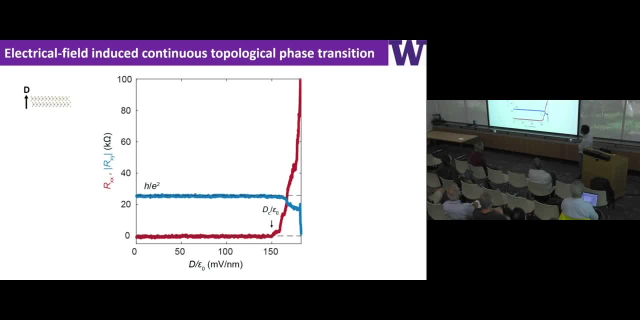 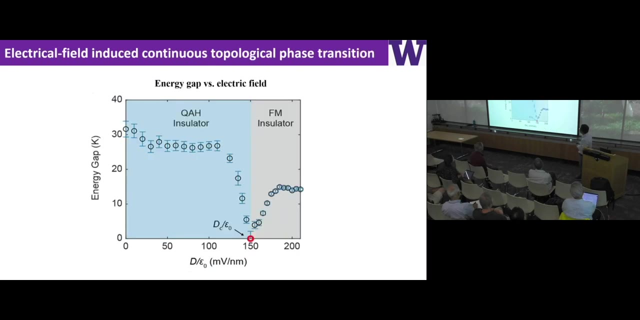 I will just skip these, But the take-home message is that we can use a large field to tune this state from this quantum anomalous hot to this insulating state which is a ferromagnetic and consistent with a couple of theory predictions. I'm going to skip all these, actually. 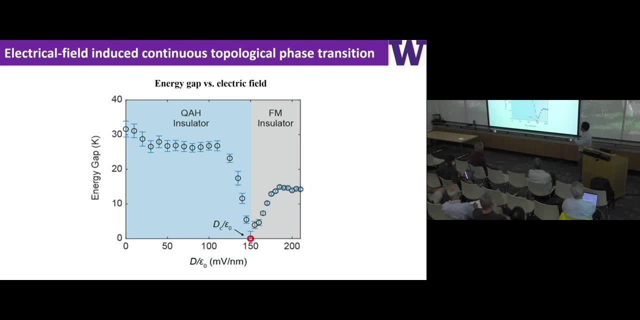 because, for the interest of time, This next part I'm going to show you. What do I mean here is that we measure the thermal activation gap of this quantum anomalous hot insulator as a function of a large field. So we see that this thermal activation gap 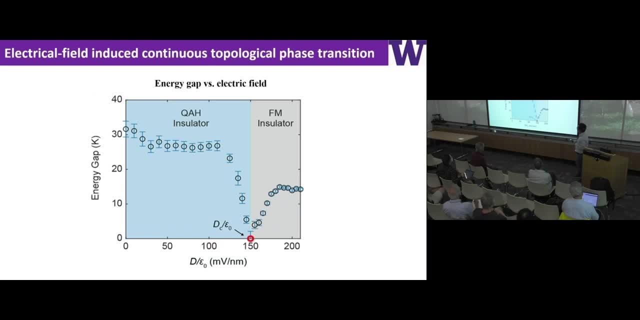 is about 30 gallons. As we tune this large field actually, the gap eventually shrinks and vanishes, then increases again when it transitions to a ferromagnetic insulator with topological trivial. So this just shows you how we can use the large field to tune the phase transition. 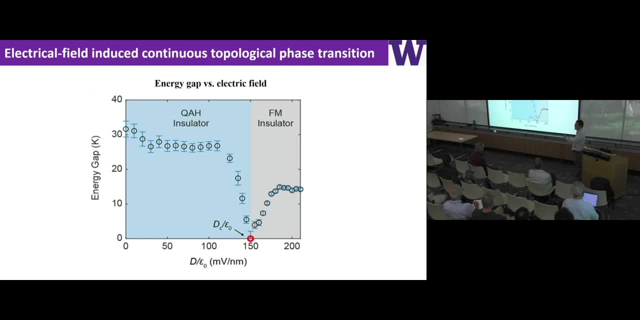 from one gapped phase, which is topological, to another phase, which is topological, trivial, And it consistently, is all a theory prediction you can think of: right, The gap must close. Okay, so now I'm going to shift gear. 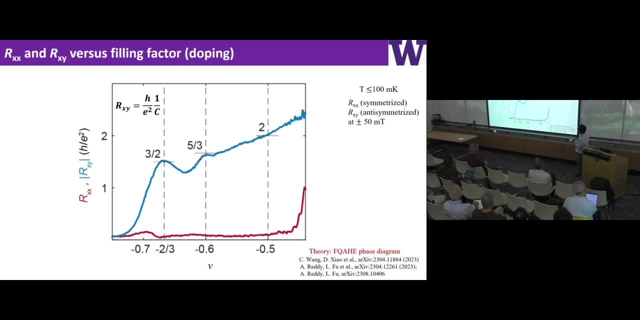 to this fraction quantum, anomalous, hot state. First, I'm going to show you the line cuts of these Rxx and the Rxy as function filling factors And we see a few humps right corresponding to this fraction filling two-thirds, three-fifths. 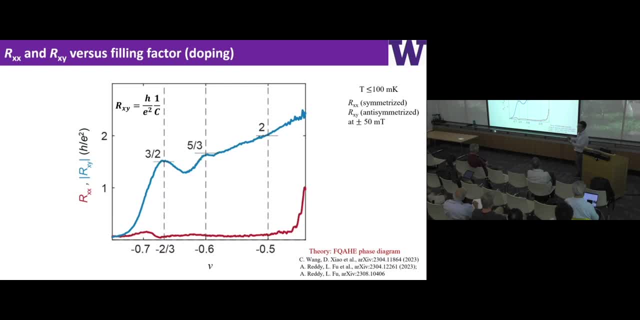 and this, basically, is a signature right of this fraction: quantum anomalous hot state. Another interesting feature is that you see the Rxy actually linearly increase as a Kerr identities and across almost two h of e squared at the filling factor minus one-half. 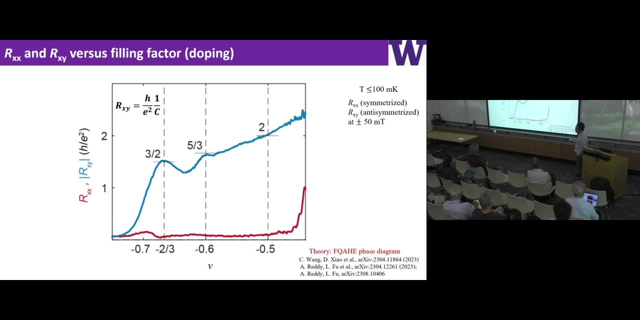 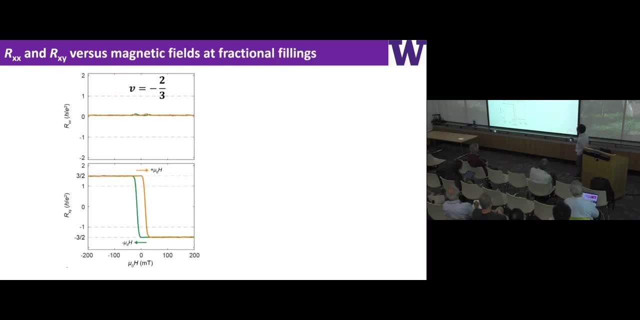 So this shows that at the minus one-half the state is probably compressible. It's distinct. finally, It's a two-thirds or three-fifths state, All right. so first thing is why we can do the same measurements, perform Rxy measurements as function. 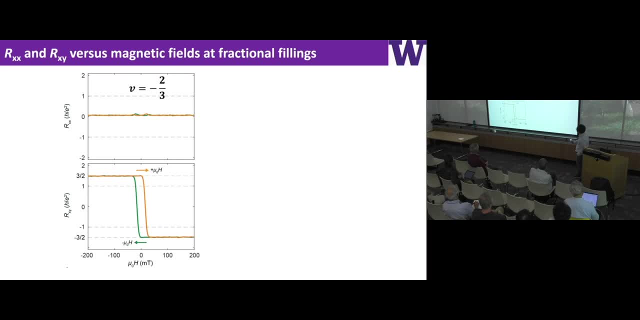 of magnetic field and Rxx. you will see this: Rxy is pretty much quantized to the, you know three-half with nearly vanishing Rxx. So the quantization is about one percent okay, And we can also do the same measurement. 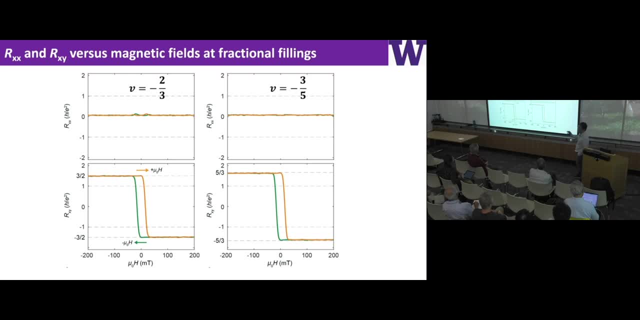 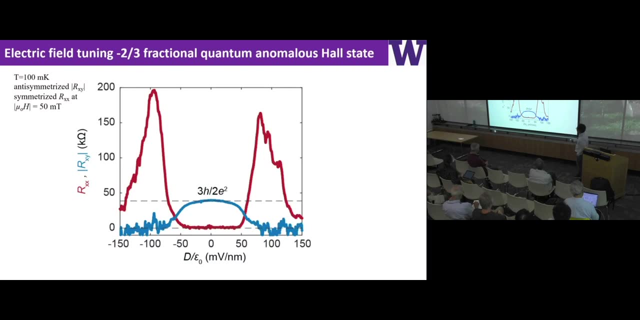 for the three-fifths states and the quantization is about three percent. And we can also tune this electric field to control the phase transition from this fraction quantum anomalous hot state to a topological trivial state. What I show you here is electric field. 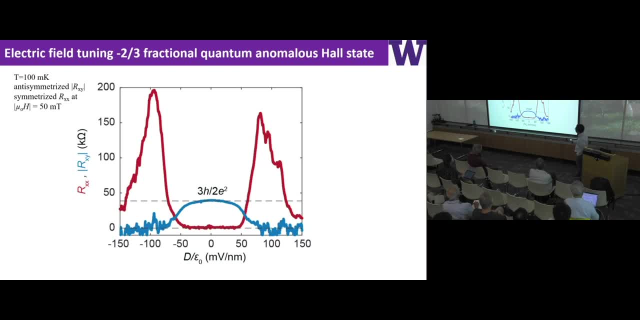 and the blue curve is Rxy. right, You see Rxy more quickly drops and it vanishes. And we see the Rxx initially was nearly vanishing. The increase seems like to a insulating state, then drops again, seems like to a metallic state. 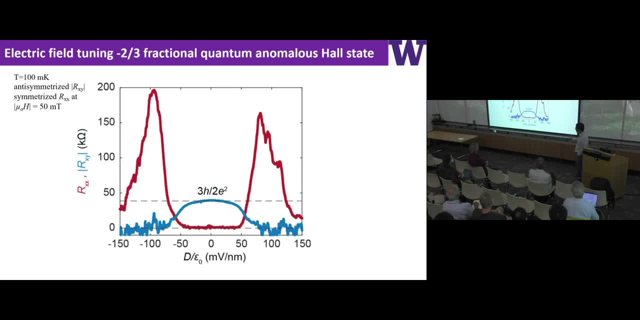 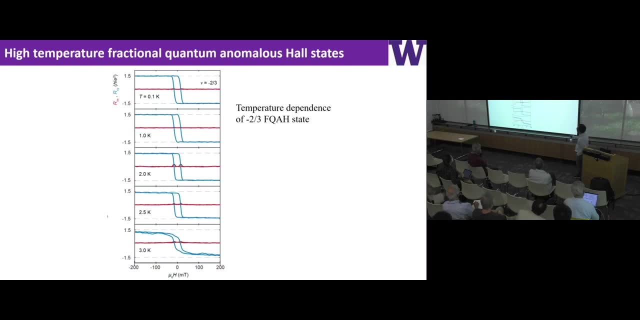 So we don't know exactly the nature of this state. This is something still on the study. I still want to emphasize: right, this feature is high temperature. So what I show you here is the data of this two-thirds state as function of temperature from the top to the bottom. 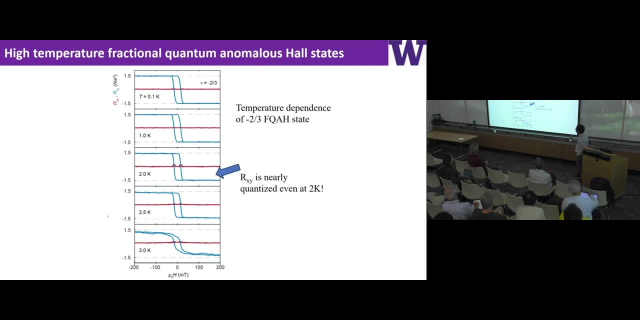 at increased temperature from 0.1 Kelvin to 3 Kelvin. So what I highlight here is, even at the 2 Kelvin the state is still nearly quantized right. So this shows it's basically telling you the energy gap is pretty large. 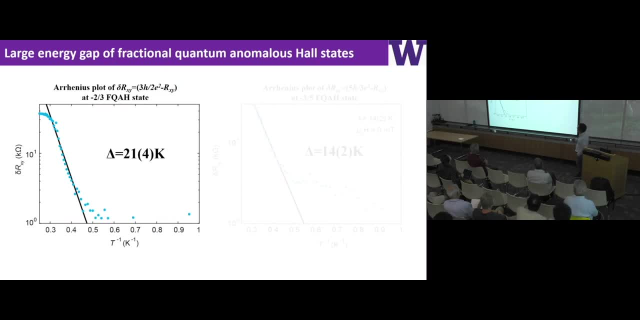 And we can perform these thermal activation measurements again and they give us this gap of the two-thirds states is around 20 Kelvin, which is 3-fifths states is about 14 Kelvin. But I have to warn you that these thermal activation gap measurements 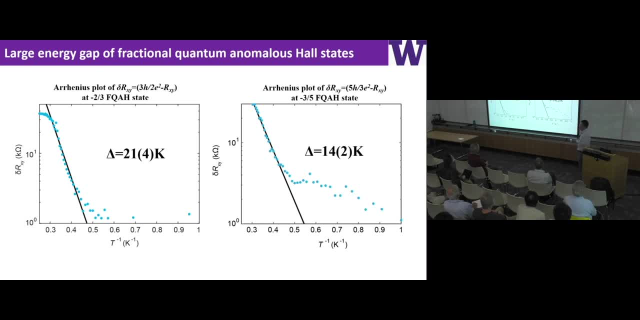 is not very accurate, right? Yeah, Leon is shaking his head, But I will tell you you can trust this number very much, right? But those thermal activation gap is not very accurate. But the take-home message is it's a large energy gap. 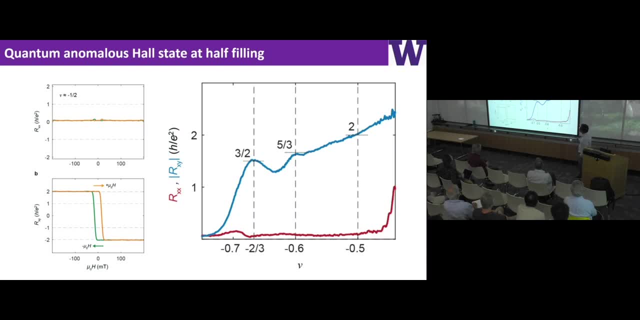 All right. So last I want to touch upon is this one-half state. We can do the same measurements, right? So this is a Rxy S-function magnetic field and it looks like a quantized. but don't be fooled by this plot. 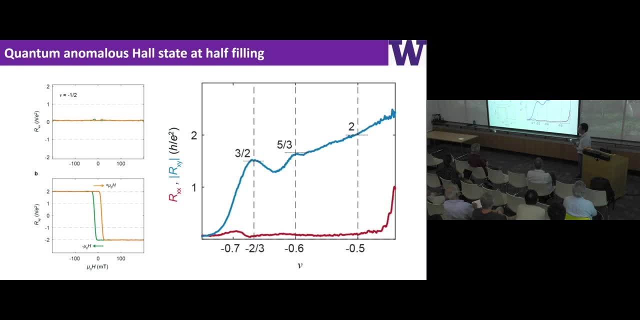 This doesn't tell you the state is quantized. It just tells you there's anomalous Hall signals And we saw the anomalous Hall with Rxy is 2 Hv squared. But if you look at these Rxy S-function feeling factor right. 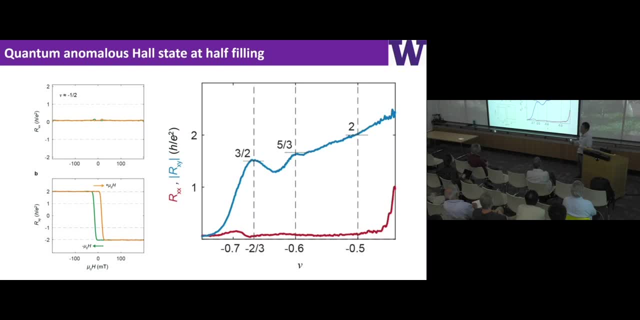 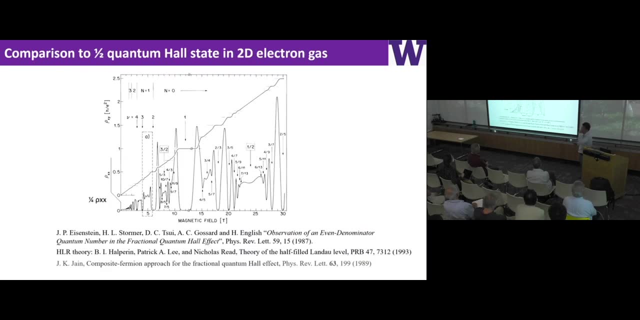 you see it's almost linearly increased. It means the state is compressible. okay, So it's not in a fractional quantized state or in a quantization. So what's going on? It's small, but we can. I'm an exponentist, right? 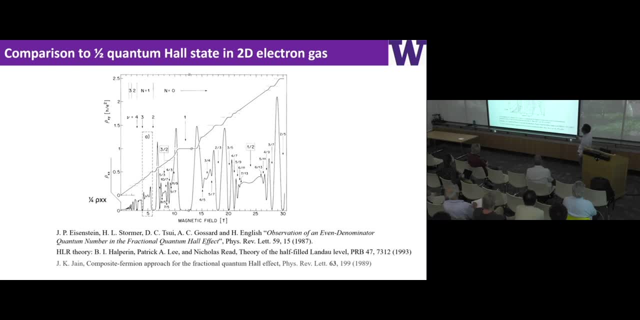 I'm kind of superficially compared to what's already been done in the past for a 2-D electron gas system. So this beautiful data, much more cleaner than what I show you, is that if you focus on these minor, If you focus on this one-half feeling S-function magnetic field, right? 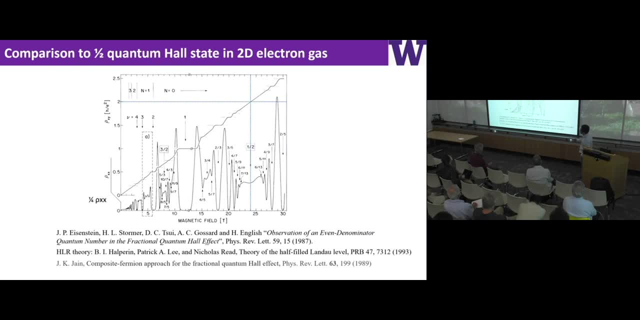 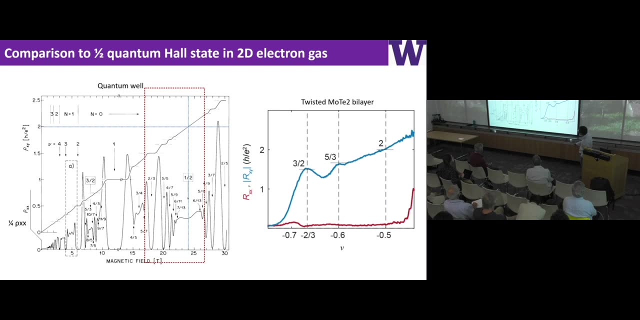 you will see this Rxy is about 2 Hv squared. Now if I compare these two data, if I look at these data from 2-D electron gas first, right, as I turn the magnetic field equivalent to the feeling factor, you see the first bump to third state. 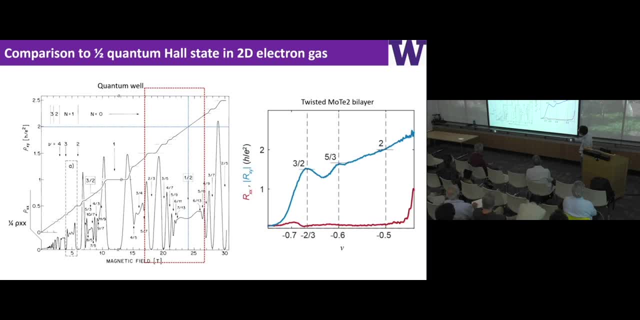 second bump through third state, some little bumps, then linearly increased. okay, This really looks similar to what I have here: right, One bump, second bump, then linearly increased. So there could be some kind of you know. 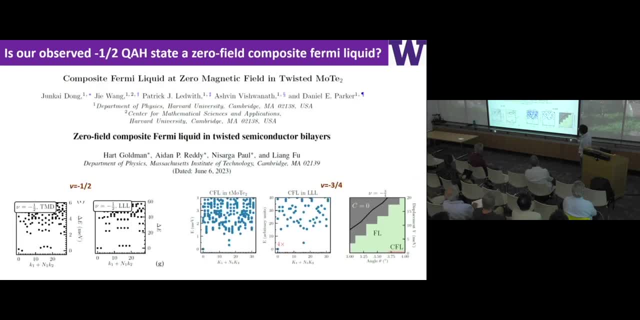 intrinsic connections between these two phenomena And when we have the data- and I'm very happy to see that there are three prints on the archive. Well, I didn't tell Ashton or Liang my data at all. They don't know my data. 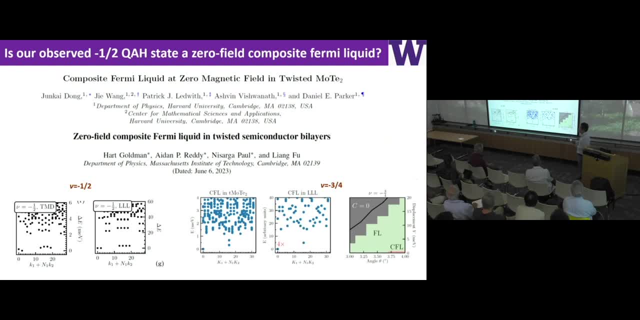 And I don't know their theory as well until it's come out in the archive. So what they say is that these minus one-half quantum-animal Hall state is actually a zero-field composite thermo-liquid in this MLT2, okay, So well, we have some signature right for that. 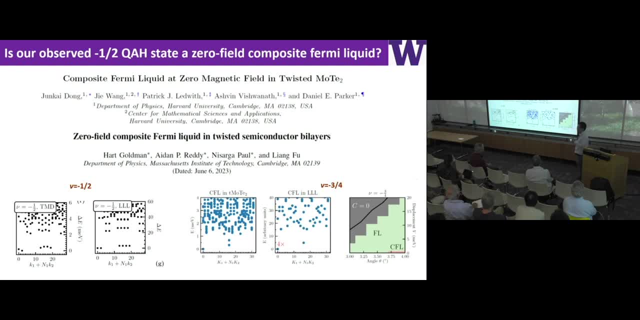 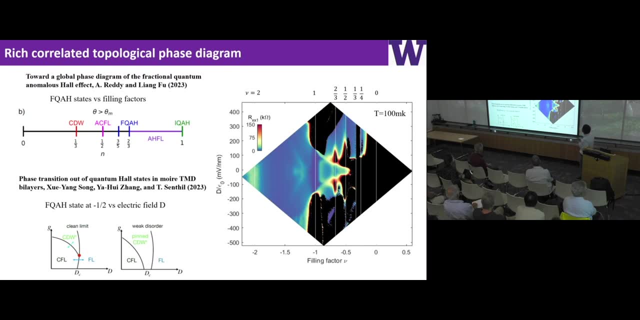 And recently we did some other measurements and also support these interpretations. Okay, So finally I will show you. you know, the phase diagram I showed at the beginning was kind of a small part of these whole measurements, But you can see that what I show you is R-X-X right. 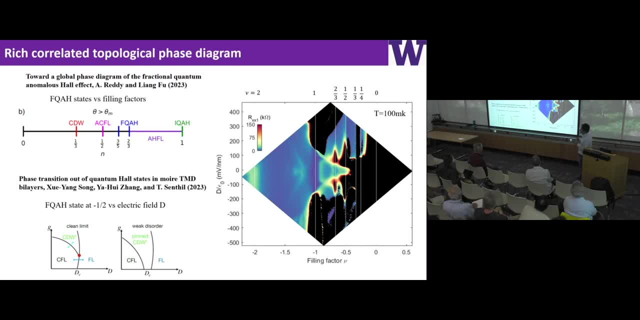 as function of large field, as function of infine factor. There's lots going on in this plot And it's very rich phase diagrams. For example, right, at least one-third state, what we see is a C-W state. It's not a topological. 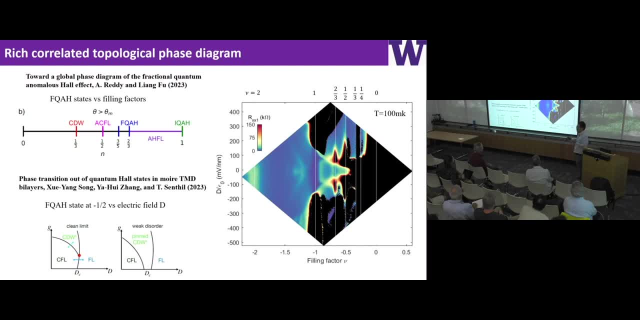 And many of you may wonder right why one-third seems very robust. Why not a FQH state? Why is it a C-W? Honest answer is: I don't know, But you can ask Liang Fu. He has these calculations. 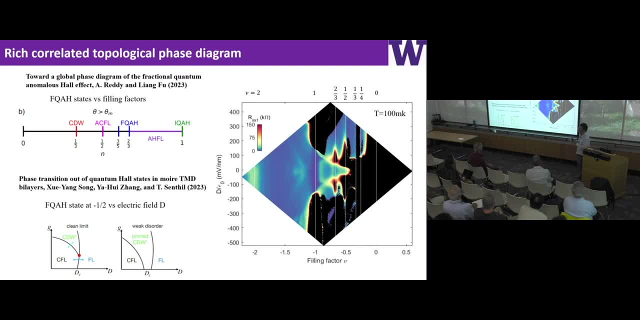 But the calculation is done after the experiment, so you have to be careful. what it means, right? So what they show is when the theta is away from the optimized twist angle. this is the phase diagram he predicts, right, You have one-third C-Ws. 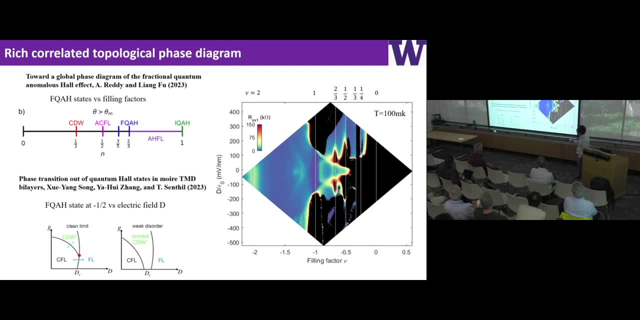 One-half is composite from a liquid, Then you have a two fraction quantum anomalous state If at the optimal twist angle, there's a lot more states going to show up. So that's what we are looking for right now, And there's also interesting predictions from Sento, right. 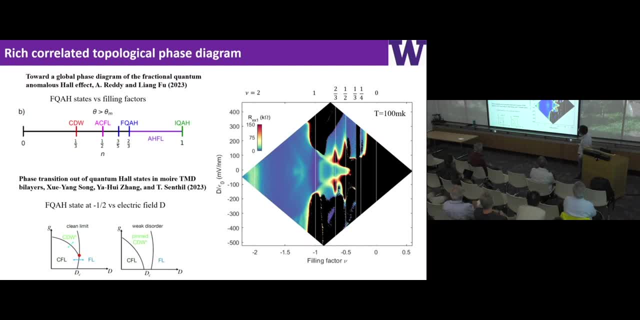 how you can tune this large field and find this composite from a liquid to a firm liquid state. But what we can see here, this is one-half state right. When I tune my large field, you will see this R-X-X actually will dramatically increase. 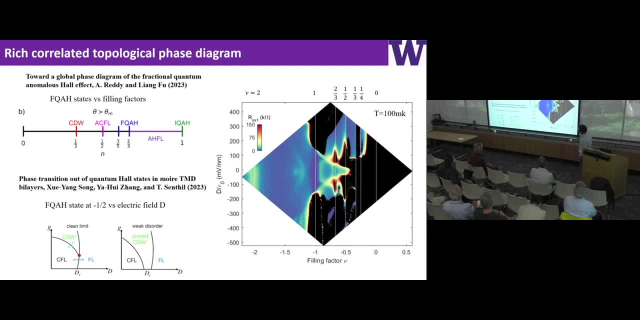 then drops again at the very end. This is a very high, large field. So this sort of is suggesting we have a transition from some metallic state to an insulating state and to some kind of metallic state again. So this might fit into Sento's, you know. 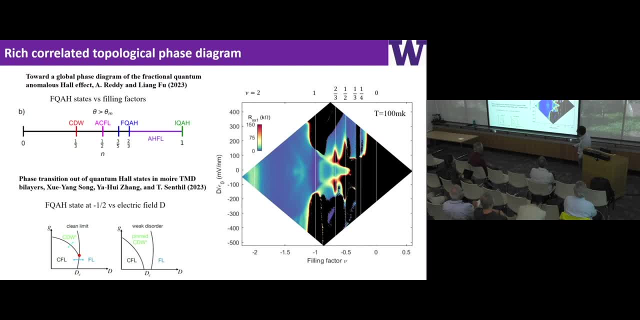 this picture which he suggests there might be a weak disorder in the system. So in the intermediate large field regime there could be pain in the C-W state. All right, The take-home message is: there's a lot of interesting things. Last one, I think actually very important. 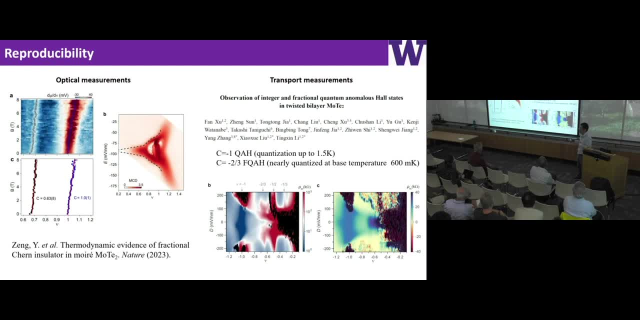 is this phenomena? I believe right is that the normal T2 system is highly robust because there's already, you know, a couple of groups of 10 very similar results. So the first one is from Cornell Group. They did these external sensing measurements. 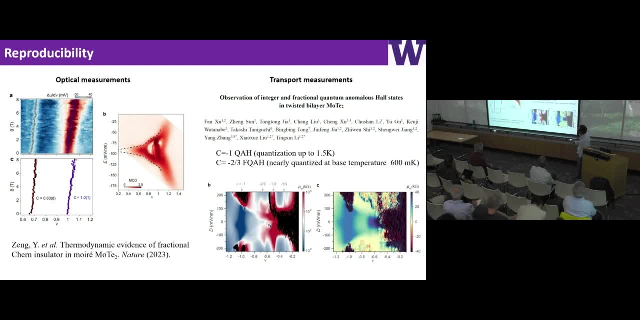 They observed this fan diagram, very similar to our optical measurements, then observed these two-thirds fraction quantum-anomalous state- And the other is a transport measurement- and found a group in China. They also observed these two-thirds fraction quantum-anomalous state. 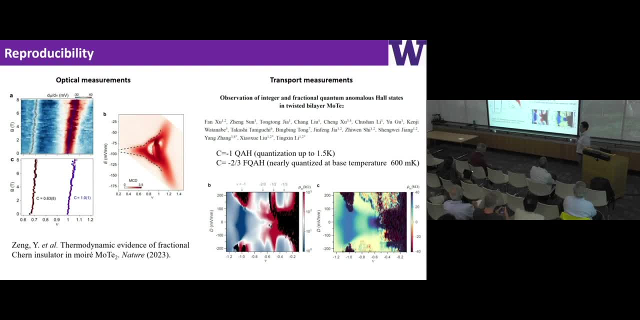 But the three-fifths state has not been used yet. You know, I think, from my own experience is that this state actually is very fragile and it has very high sensitivity to the quality of the samples. One example, right if you look at these: 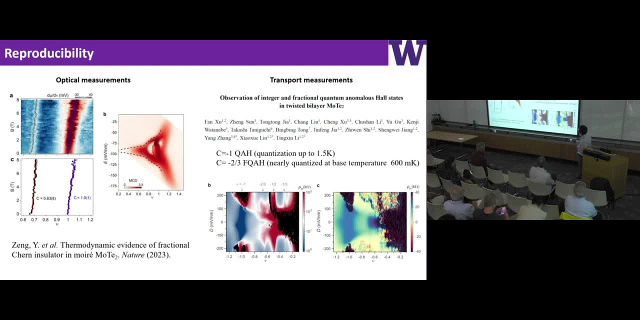 quantum-anomalous state from these transport measurements. you see, its quantization is up to 1.5 Kelvin, It's not 8 Kelvin as I just talked to you, right? And this minus two-thirds FQH state actually is not fully developed. 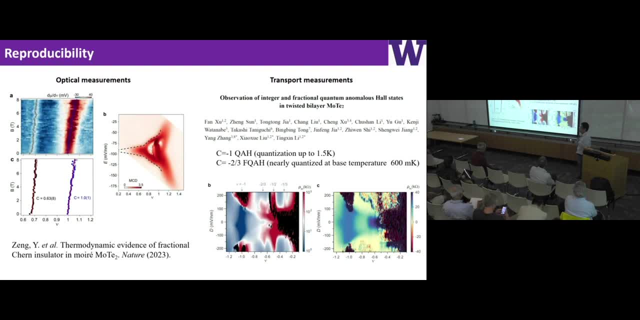 even at 600 millikelvins. That was another 2 Kelvin I just told you. So I think this probably has something to do with the sample qualities, But the overall take-home message is that I think the system itself is very robust and, you know, could be good news. 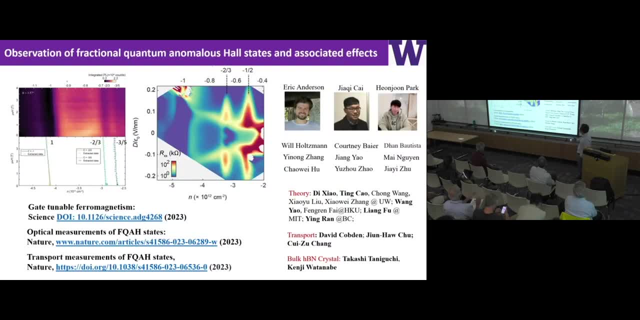 for the experimentalists. Okay, so here's my conclusions. I will leave it here, but I would like to thank my students, These three students. they did the most work, And I thank all the theorists and my colleagues for help in the transport. 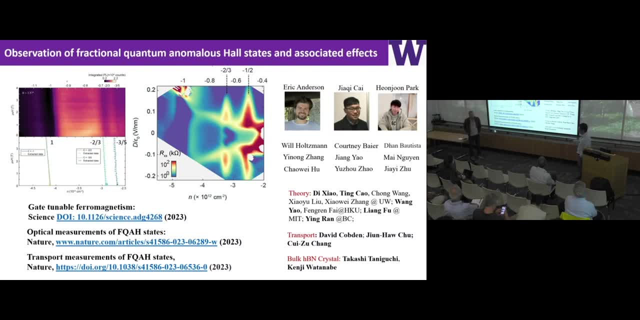 and also the crystal from the Japanese group, And thank you for your attention. Okay, thanks for another great talk. We can take some questions. Is there a reason you saw these fractions only on the whole side and not on the electron side? Yeah, so first you know. 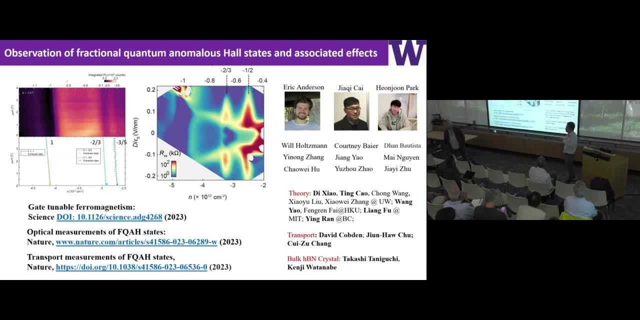 because it's a light assistant. so there's no electron hole symmetry, right? Because it's a light assistant, Very different from Kronen Hall. The second is It's a semiconductor And the second is: why a whole band? The honest answer is: I don't know. 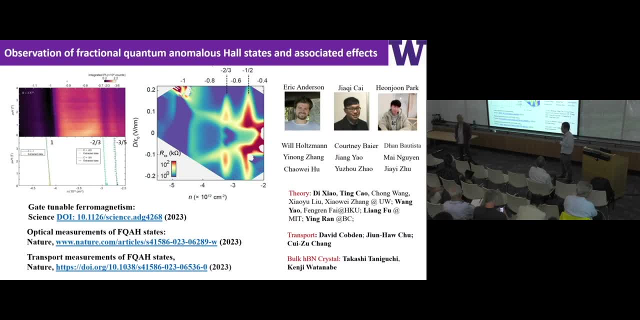 But I can tell you what I think. what's happening is that there's a very strong spin of the coupling induced. the splitting in a whole band. It's about 200 millivit. Okay, So for the conduction band, the spin of the coupling is. 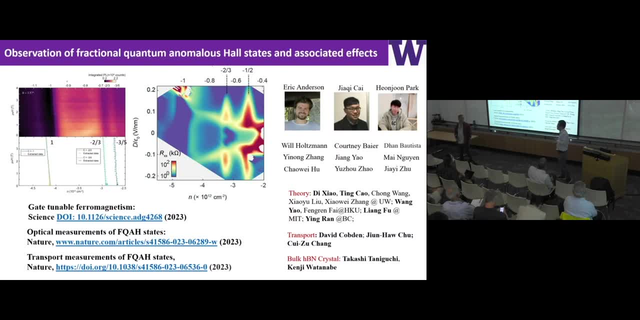 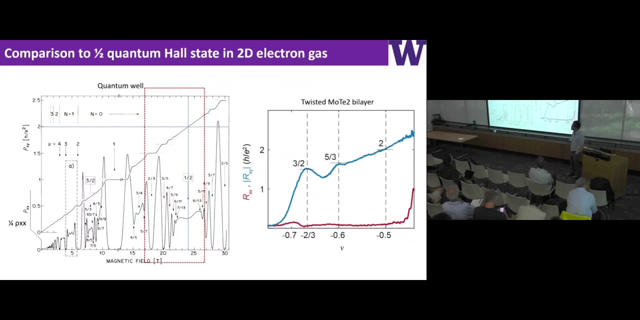 for a week is about 30 millivit or even less. So that might be the reason. yeah, If you go back to the slide where you're comparing it to the gallium arsenide plateaus, why does the Rxy come down in? 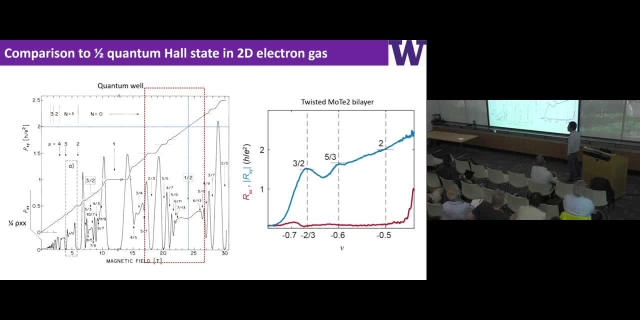 I mean, that's not a feature. Excellent question, Yeah, But why does it come down? This actually says the system has something new. So I'm going to repeat what Leon. he told me. okay, So what he thinks: there's a phase transition from the two-thirds state. 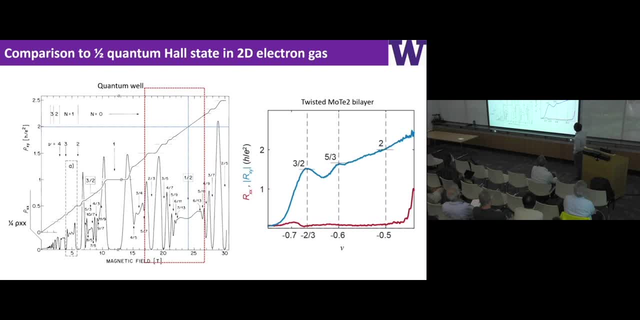 to the rest, you know feeling factors. So if we believe that minus one-half is a composite liquid state, a zero-mana field, then this composite liquid state, actually it's a parent state for many states around these feeling factors Okay. 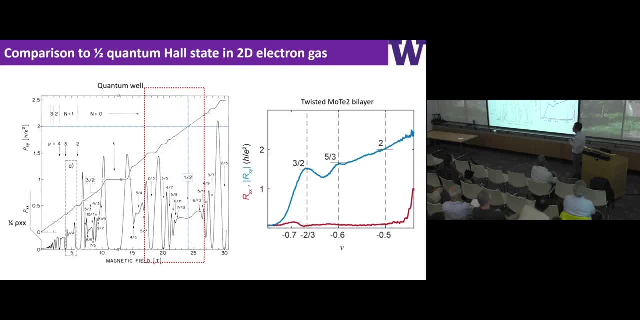 So what this dip, what it shows is, if we take you know, what I told you is correct. what it says is that the two-thirds state doesn't share the same parent state of these three-fifths state. Yeah, that's what it means. 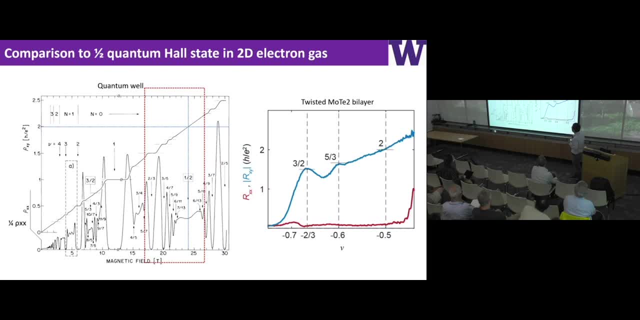 I think Ashwin is here, right? Maybe he can tell you more. He was here, He just left. Yeah, I think he. Oh, you're here. Okay, I saw that you tried to avoid the question. Anyway, so that's what I learned. 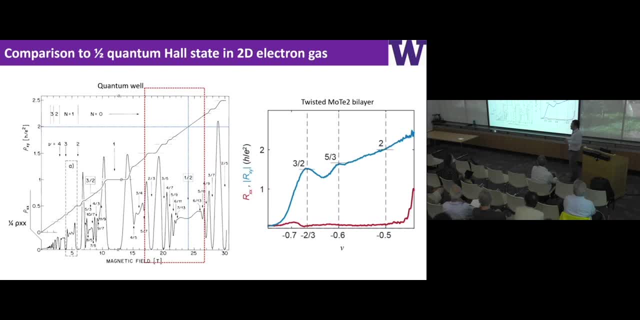 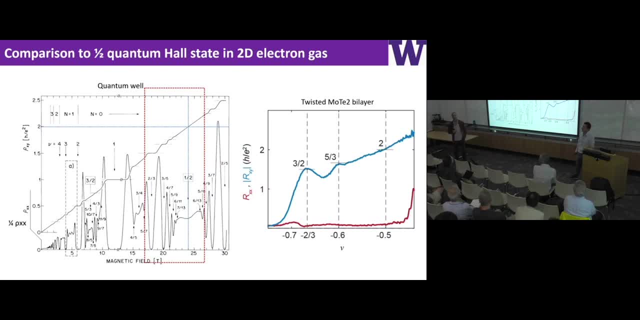 Thanks, Thank you, Thanks, Thanks, Thanks, Thanks. Yeah, In the range from two-thirds to one there's a lot of MCD signal that seems from the Trump home better than the RxY home signal. Yes, Excellent questions. 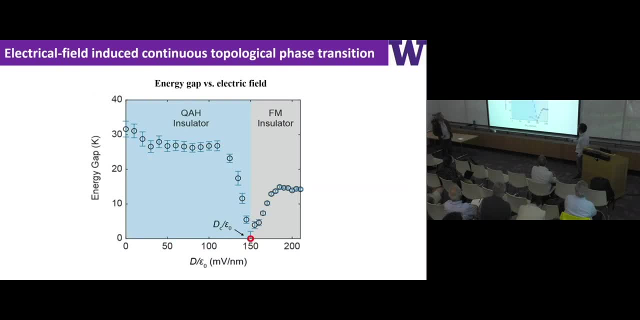 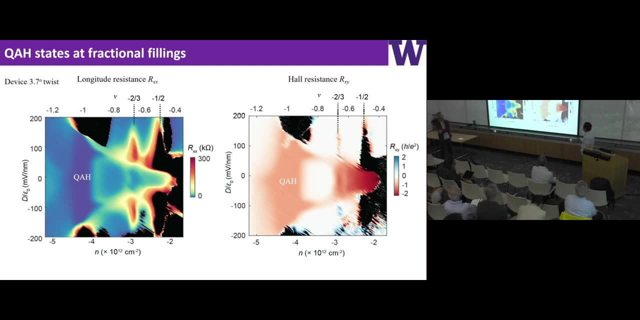 Can you repeat the question? So this is a very good question. Let me just look at this. So the question is that in my MCD measurements, right my gneிsicr diprism, it's not exactly You know- from the whole face space there's a third of my United States. okay, 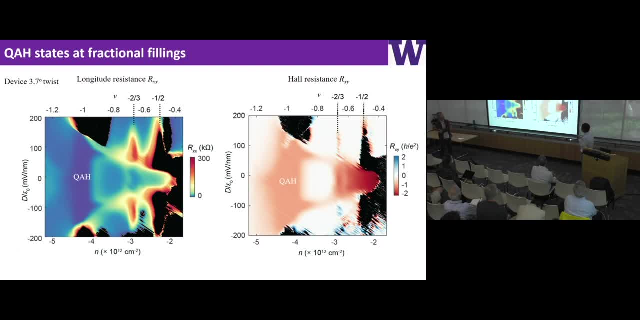 But in my transport- you look at this plot, right, Looks like RXY is very small in this regime. So that's the question, right, The question is why MCD shows strong signal but RXY is small. So if we compare these two plots, right, one is RXX, the other is RXY. 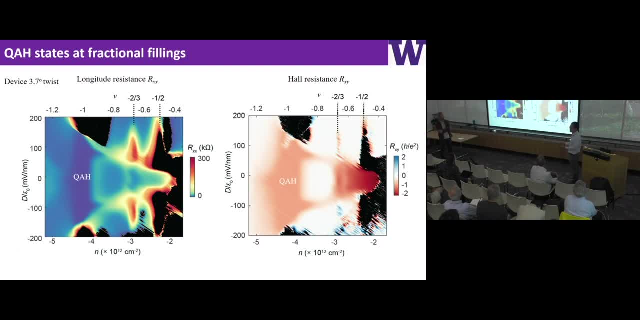 you will see that in this particular regime we call anomalous hot metal regime. okay, So RXX first is very small and RXY is also very small, But the ratio between RXY to RXX is actually not small. 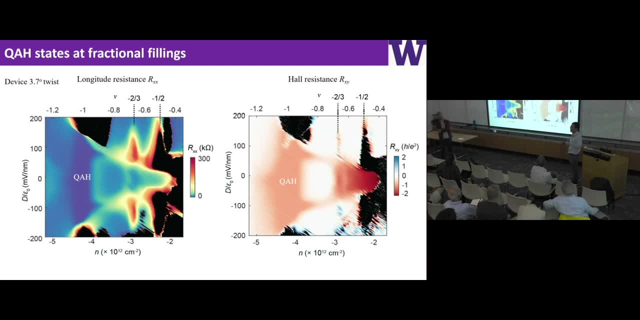 So the hot angle is about 30 degrees. okay, So this phase we tentatively assign it to anomalous hot metal regime. yeah, Yeah, Yeah. I guess another feature of MCD is that when you get past megaballon filling, 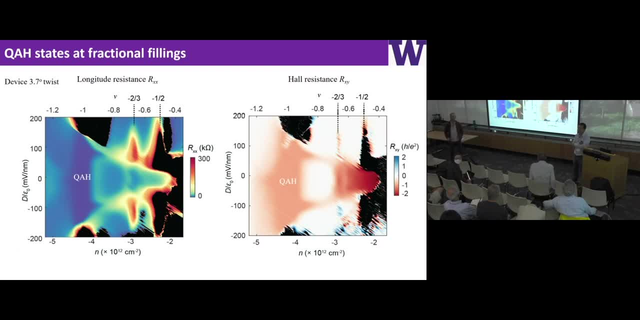 and you go like further, you have this feature that seems like it's going to be a little bit longer. Yeah, It's kind of like dispersing or defining. you know, that's what you would think of what that is. 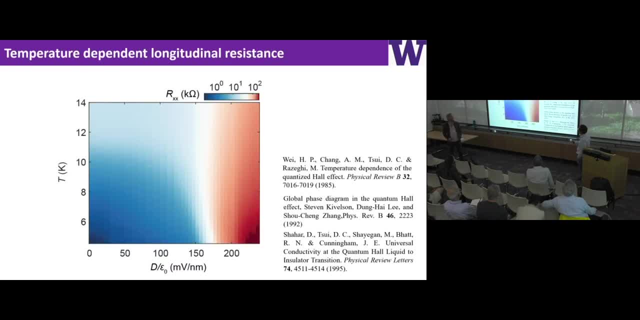 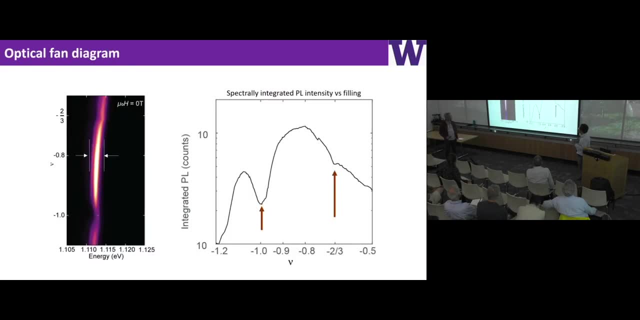 Yeah, Well, you know I didn't, let's see if I have. so we basically explained, you know, in our first paper. you know about these ferromagnetic states, okay, So what's going on there is that, first of all, it's also anomalous hot metal regime. 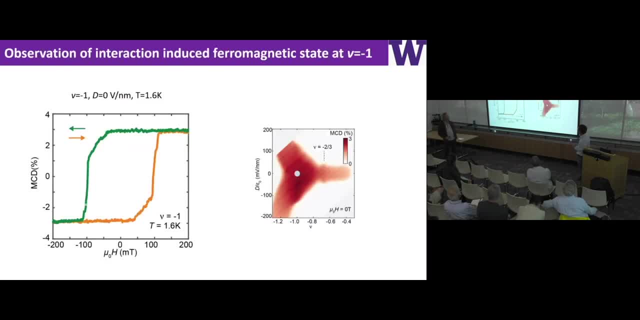 because you dope it right, So you dope it into the metallic regions And yeah, basically it's this. So this guy is actually, it's a you can. it's a ferromagnetic metal phase. That's a simple answer. yeah. 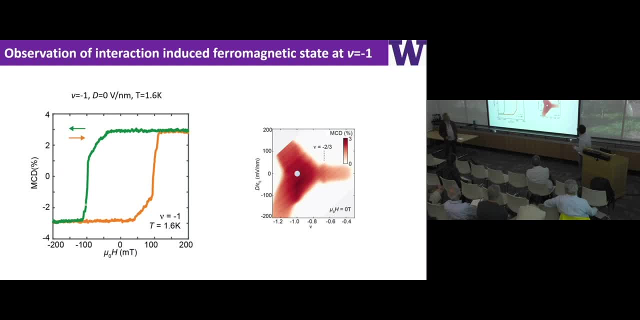 Oh, yeah, yeah. yeah, The reason is that when you apply electric fields, you're basically redistributing the electrons between these two layers. okay, And so what the calculation shows? that is, at a certain displacement field, the electron wave function from top and bottom layer is overlapped the most. somehow. 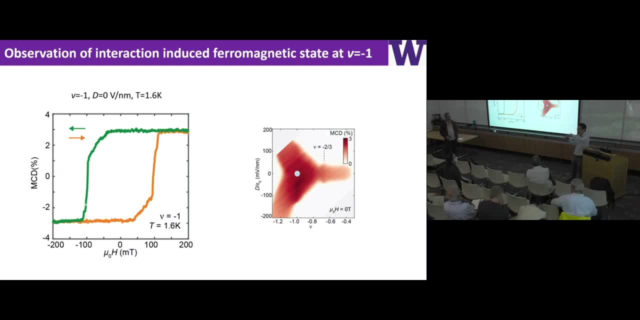 And then we need these electron wave functions. We need these electron wave function overlap to have these direct clone exchange to give rise to these ferromagnetic states. But then if you go- let's say you go even larger- imagine if you go larger. 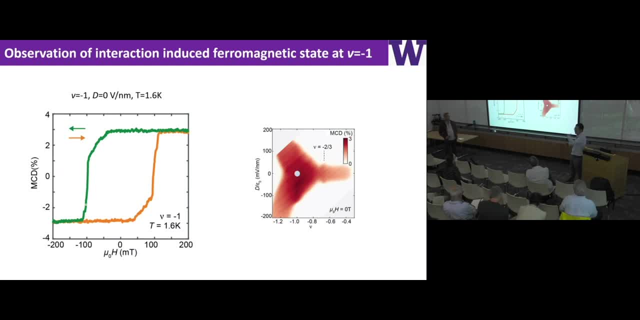 you push all the electron into one layer? okay, In that case then the ferromagnetic will just vanish because the system becomes layer polarized. yeah, Maybe I can comment on your question. Yeah, So one difference between the Gallimard-Snyder and your SysUR platform. 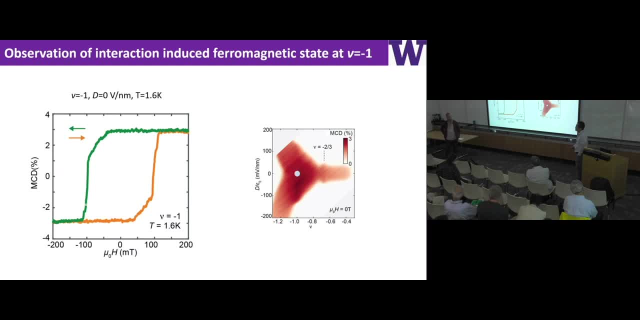 you have a dispersion. It's not large, but you have a dispersion. Yeah, So you are allowed to get a Fermi liquid which you cannot. a regular Fermi liquid. you couldn't get in a lander level. Yeah, 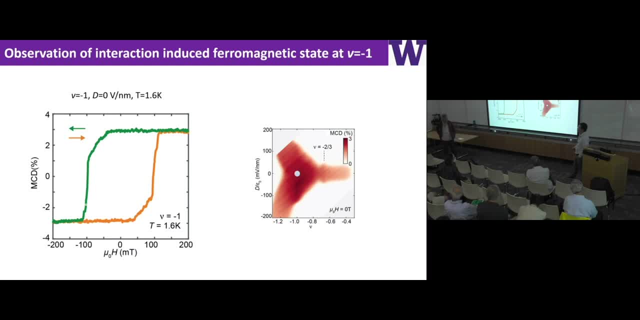 And that's competing with your fractional states, Mm-hmm. So you know, presumably between minus one and minus two-thirds, as you also suspect, you, you know, the fractional states lose the computation and you get the metal instead. 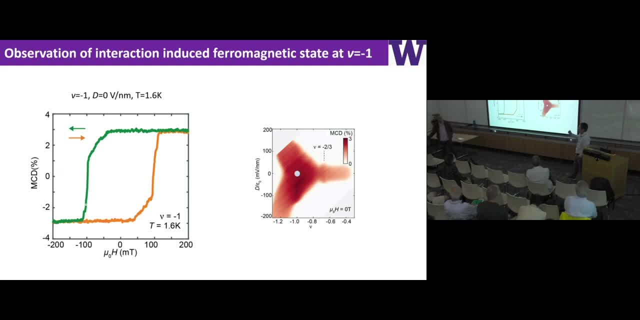 Yeah, So basically there's a phase transition to something right. Then come back to topological. yeah, Yeah, Thank you for help. Any more questions? No, Oh, okay, one more. There we go. How do you interpret the Arrhenius plots, or why are they interesting? 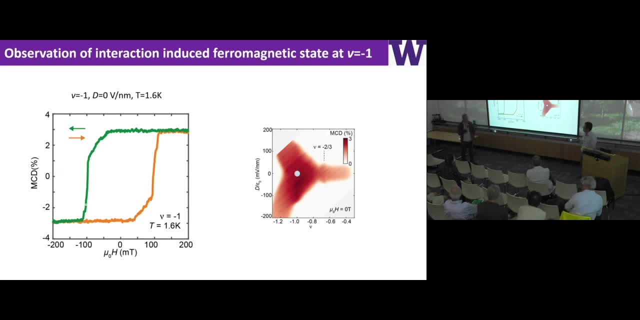 Can you repeat the question? The question, I can repeat it. How do you interpret the Arrhenius plots, and what was it and why are they interesting? How do you interpret the Arrhenius plots, and what was it and why are they interesting? 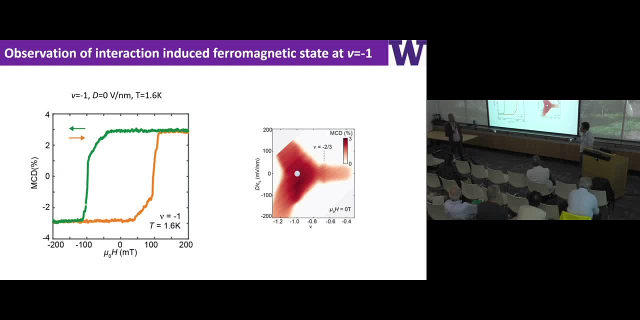 The, the, the plots for the gap, where you extract the gap, the Arrhenius plots, Yeah, yeah, How, how do we extract it? What is the significance of the? the log plots of the resistivity, Yeah, so so the plot itself is a measurement of a thermal activation gap of the systems. 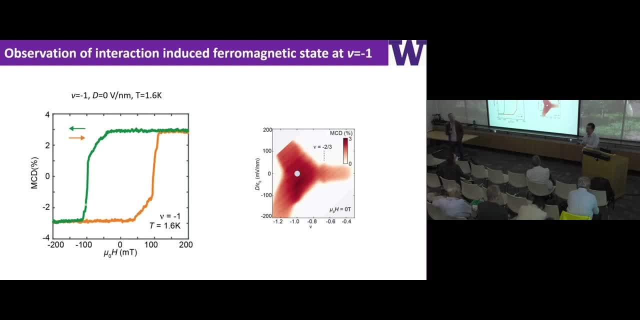 And they sort of tell you: you know- not a very accurate way to tell you what's the energy gap of my state, Because it's important, right, If a large energy gap means you can study the system at higher temperatures. So that's what the plot is. 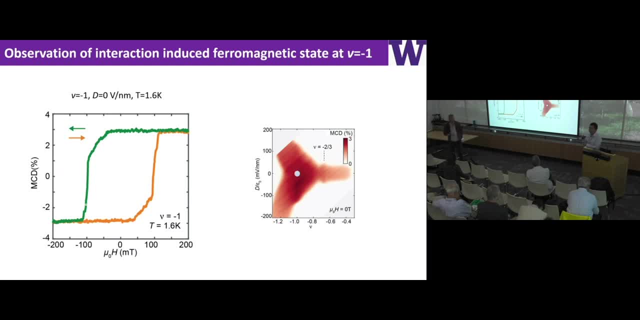 But, like I told you in my talk, is the that plot itself. you know you. just you take it, but don't trust it too much. Much more reliable results is when we match these Rxy's from human field at the different temperatures. 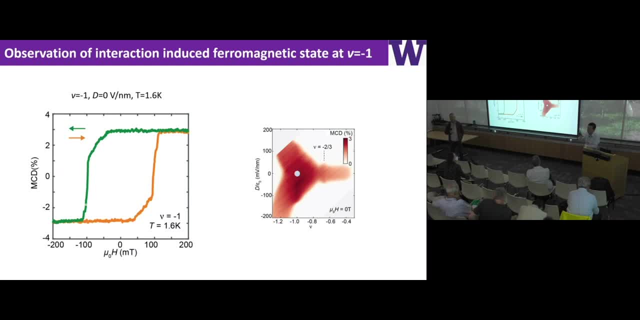 We see on the station is still there around 2.. So that one is very solid, Yeah, Oh, now we have more questions suddenly, Mike, So there was some indication that it was the CFL, some experimental indication. Yeah, I'm going to tell you October 2nd. 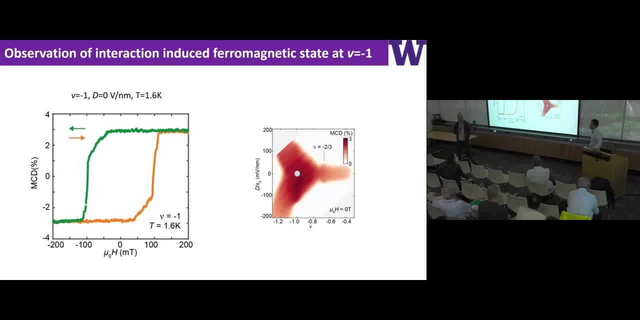 Precisely October 2nd. At what time? Mike hasn't told me the time in that time, so I don't know. Max, yeah, So this 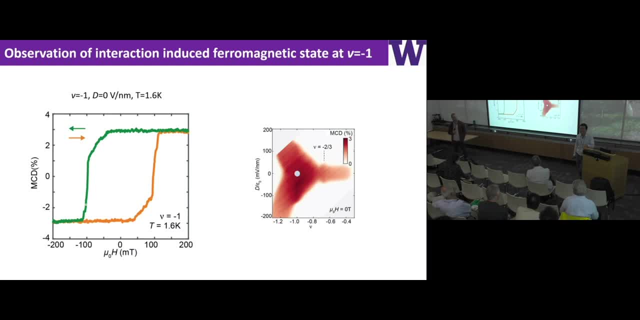 Can you repeat the question? So I think the question is in my Rxy measurements, right, It's a almost contest that the two are the same. What's the difference between the two? 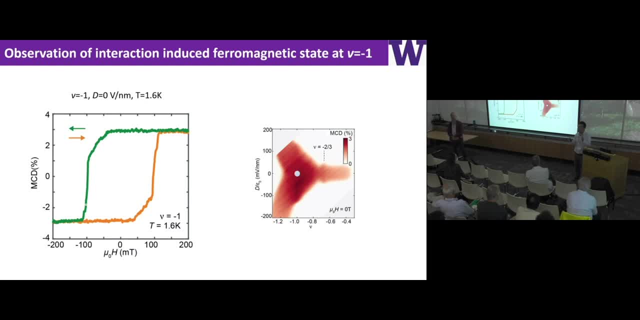 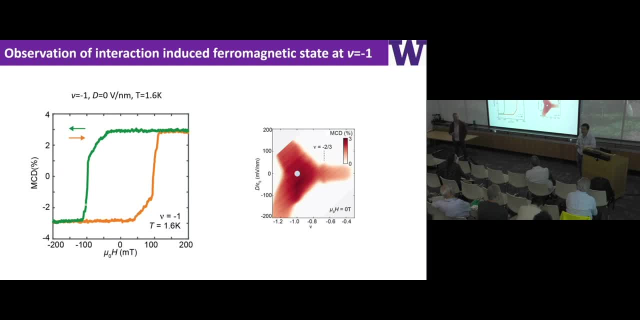 is considerably larger than the temperature at which the quantization goes away. 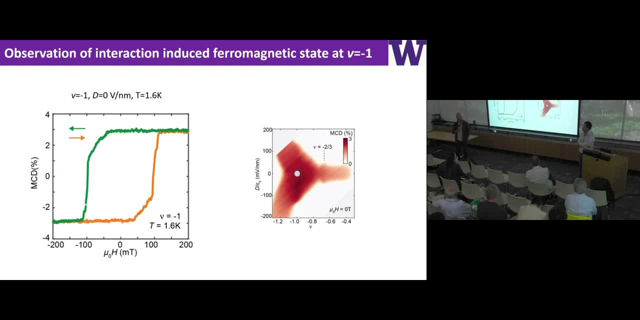 So I'm not sure if one should make too much of it. All right, one last question. So you have these sharp transitions right, like this function of displacement field. So you know, it would be interesting to study how the transition point changes with temperature. 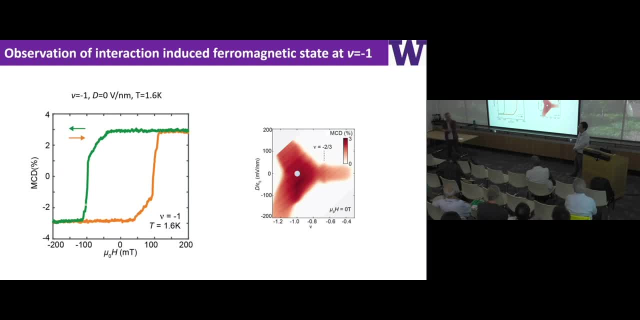 and that will give you an indication- relative entropy, for example, of the two phases. Did you look at that, how the phase boundary, how these phase boundaries change with temperature? We looked at it in terms of MCD. We did these type of measurements at different temperatures. 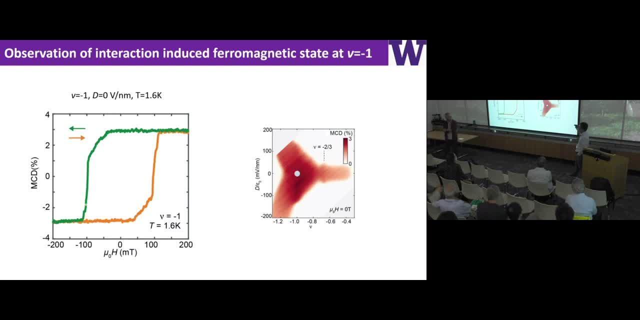 but not in the transport. We haven't done very careful measurements of the function. you know the whole map. We did it at the particular fielding but not at the map. So that's a very good suggestion actually. All right.